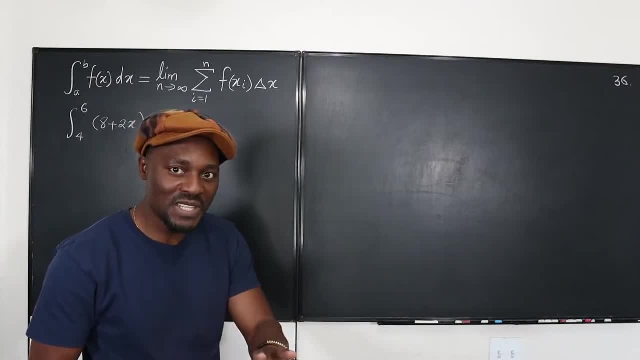 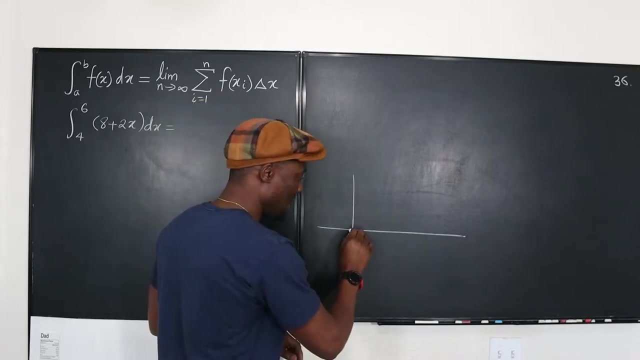 replacement. So I'm going to show you what to use to replace each of these things, just from this. Let's assume you have a function. Remember, the graph is not important, okay, to solving this, but it's important to understanding why we have to replace these things. So let's. 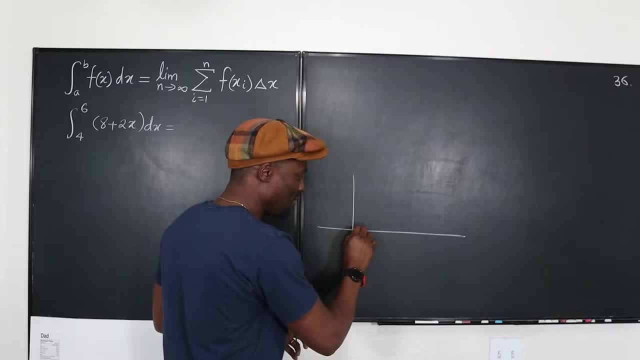 say: you have a graph. Let's just do a triangle, okay. Let's just do a straight line, Let's just do something like this And I want you to find. so let's say this is 4.. I know it's not really 4. Okay, 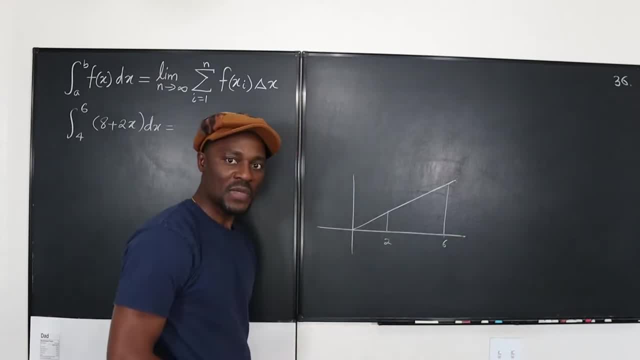 let's do 2.. And this is 6. And I want you to find the area. I know because it's a straight line. this is a trapezoid and you can use the area of a trapezoid formula to get this. 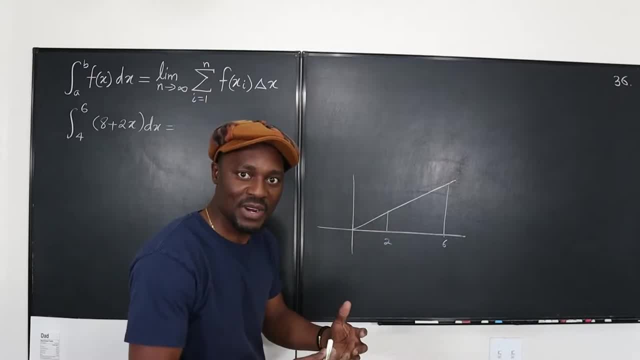 answer: Okay, you just add this to this: You take the average, you divide by 2, and then you multiply by 4.. Which is the gap from here to here. That's the area of a trapezoid. You'll be 100% correct. 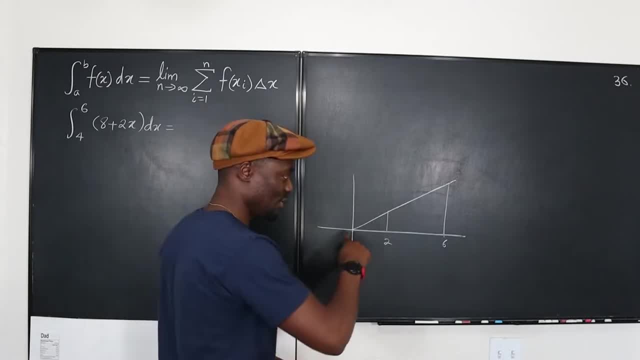 But usually in calculus you don't get a straight line, So I'm just using a straight line to help you understand the concept. So what we have is we're going to say: what is this area? Well, we don't know the area, but we can divide it into some equal parts. So 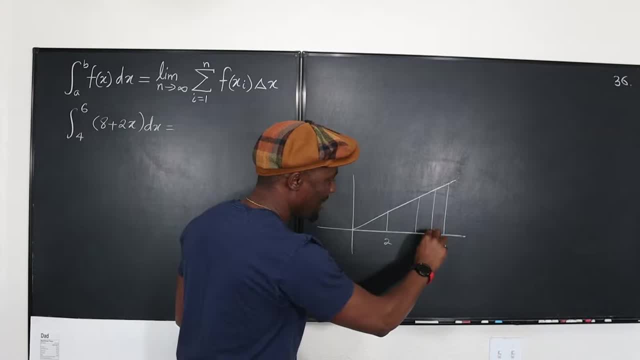 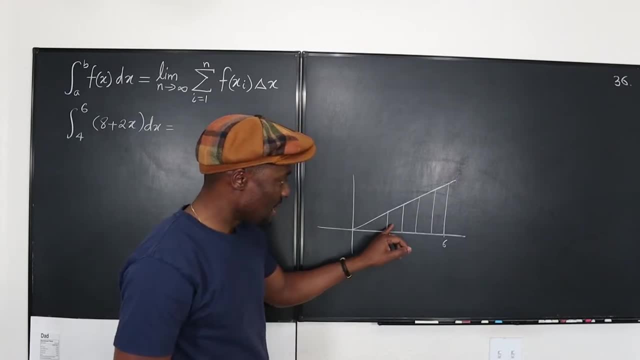 let me divide this this way. Let me divide this again. Let me divide this again. Okay, so now I can easily say that, because I have 4 rect. Oh, these are not rectangles, But now we have to assume that they're rectangles. But you can see why you have to have as many. 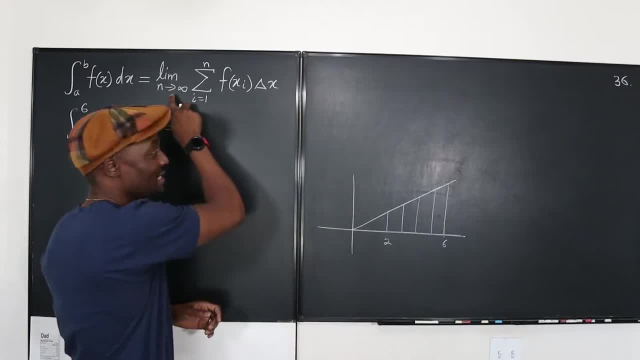 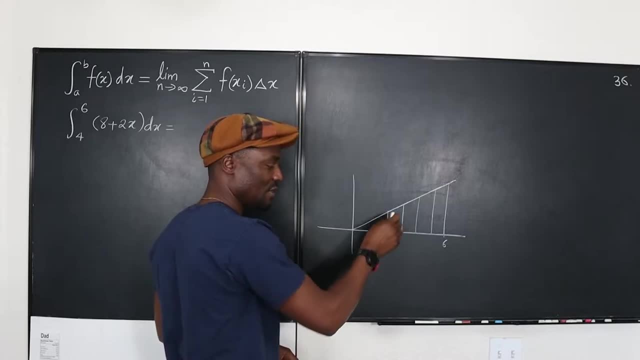 rectangles. That's why n goes to infinity. So, but let's assume we're right. We're going to assume that this side is the height of the first rectangle, because we don't want to cheat ourselves. okay, Because if you take this as the height, you'll be losing some. 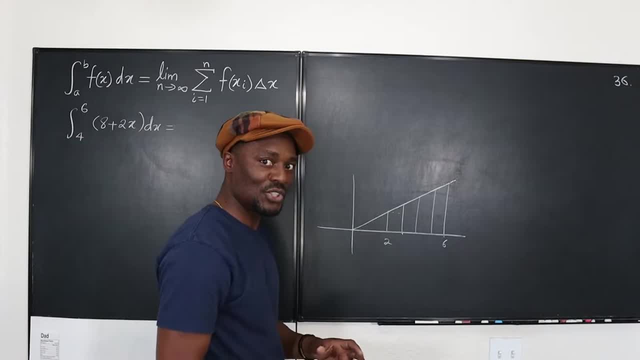 area. right, You'll be cutting off some area, But we don't want to be cheated, so we're using the right endpoint. Just follow me. So if we use the right endpoint, we know that the height of this is going to be simply 2.. I mean, this point here is going to be 2 plus the gap. 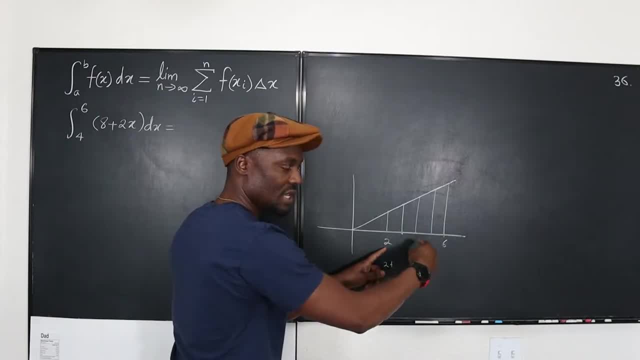 Remember, from here to here is 6.. So, obviously, because I divided it into 4, if you want to know what each of these width is, it's going to be 6 minus 2 divided by 4.. You shared the. 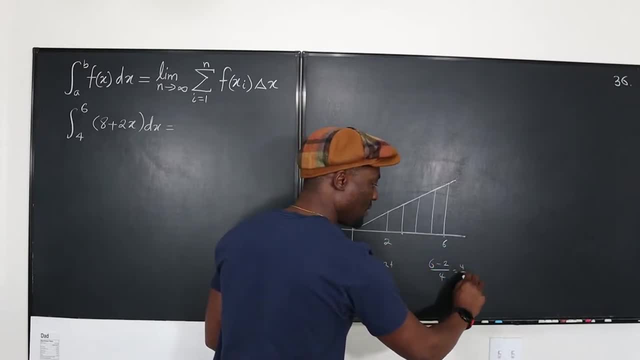 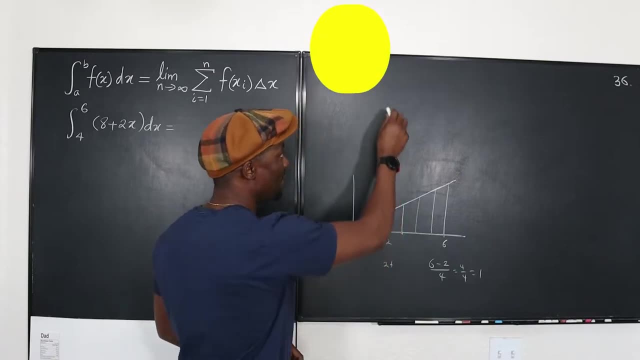 gap between 4 rect. So this is going to be 4 over 4, which gives you 1.. I want you to note what we just did here. So now, if I want to find the area of each rectangle, the area of each rectangle. 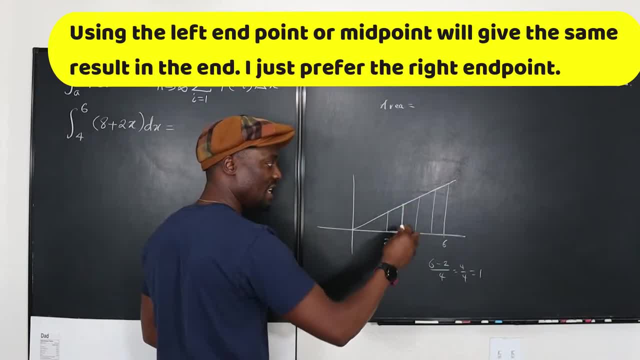 is this times the height, right? Remember, I'm taking the right side as the height. I don't want to take the left side, because I'm going to be cheating myself. So I want to gain some height, okay. So what I'm going to do is say the area is going to be this width. How wide is this? 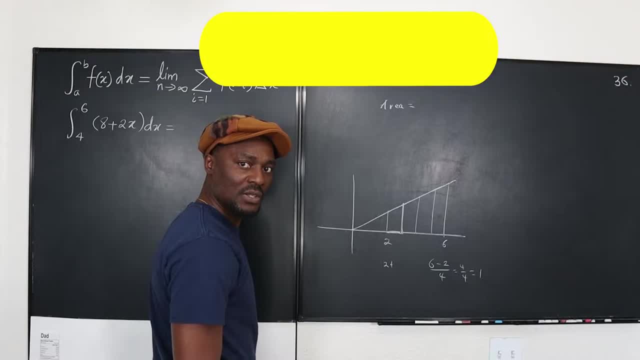 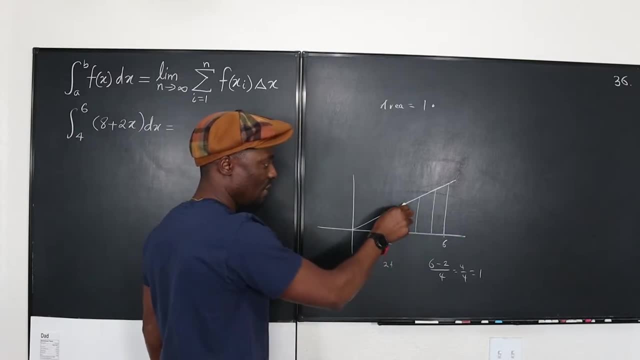 It's just 1, okay. So the width of this is just 1.. Area is 1 times How tall is this? Well, I don't know how tall it is, but I know if I go on the graph I can trace this to. 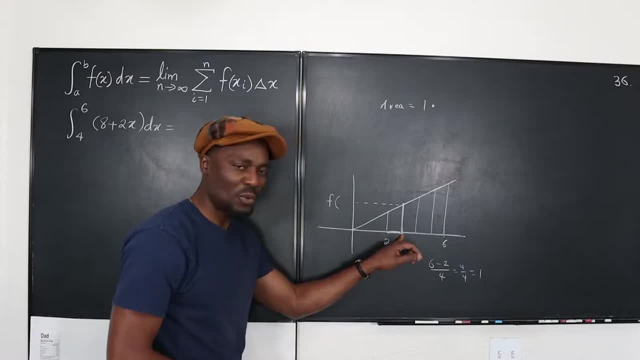 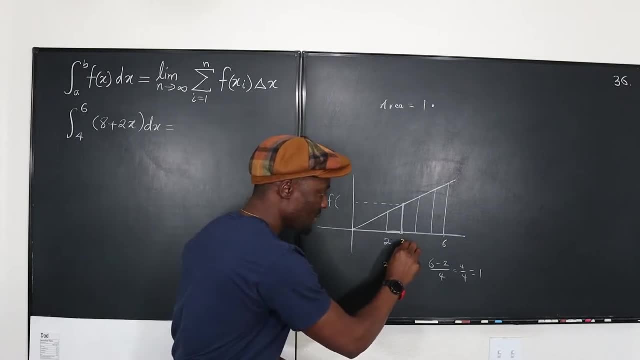 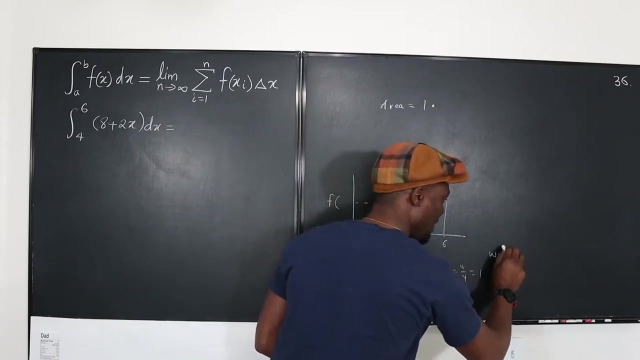 the value of the function at this point. Well, what is this point? This point is 2 plus 1, which is 3.. 2 plus 1, okay, Okay, Which is the width. So the width of each rectangle, the width of each rectangle. 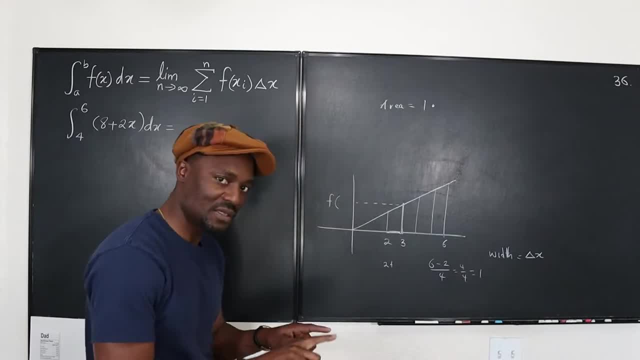 is what we call delta x, The width of each rectangle. it will be the same because you divided them into, divided this space into equal parts. okay, So we're using just 4 rectangles, So the width is going to be delta x. And how did we find delta x? We said we're going to 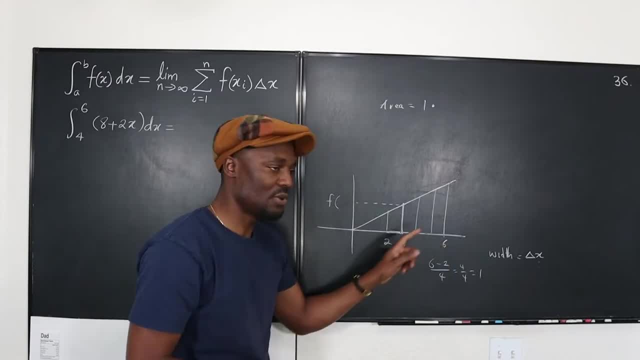 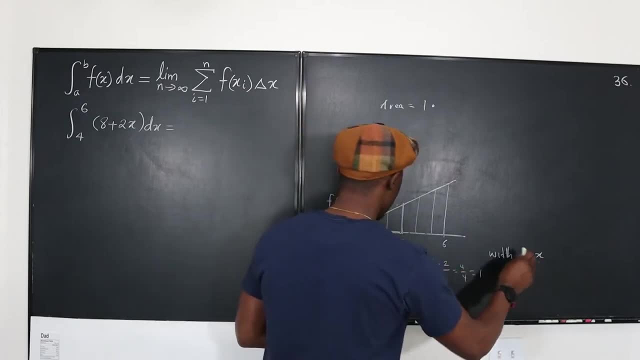 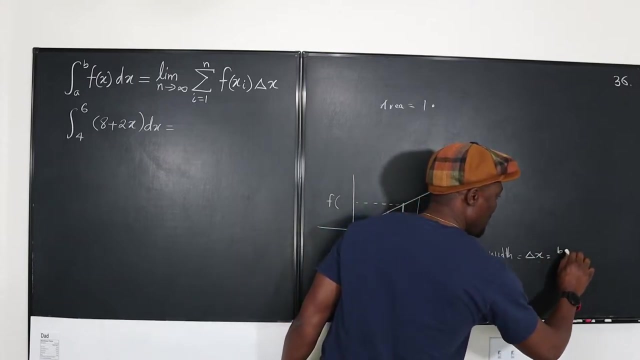 subtract the beginning from the ending and divide it by the number of rectangles that we want to use. okay, The beginning subtracted from the end, which will be, in this case, it's going to be b minus a. This is the beginning, This is the ending, So it's going to be equal to b minus a divided. 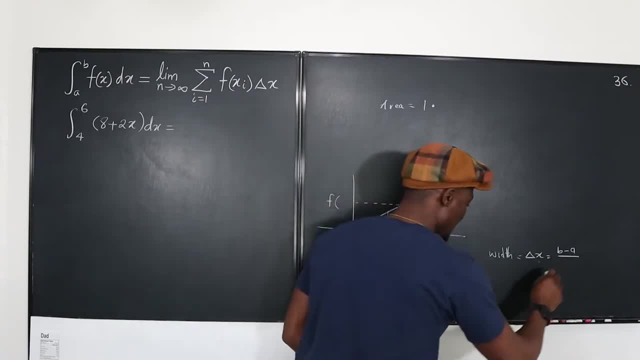 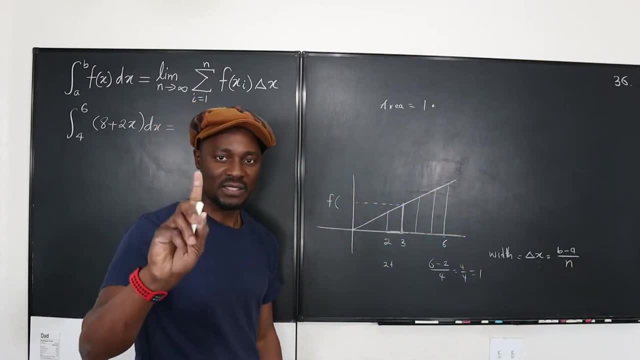 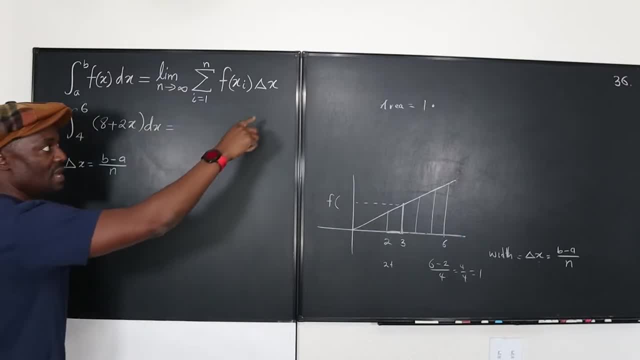 So in this case we haveيرة x, delta x minus a over n. In the case of this problem, of the problem of the delta x, because we're using so many n's, we don't have a number for it, but we know what our b is, we know what our a is, because 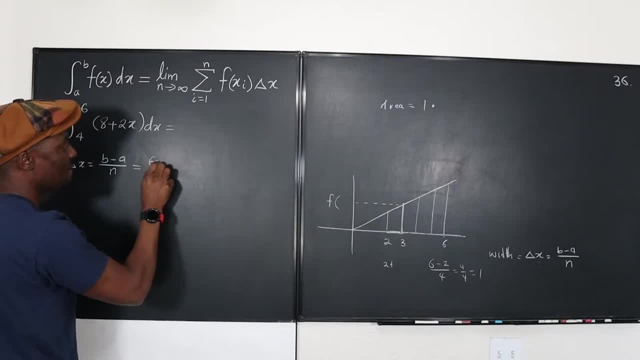 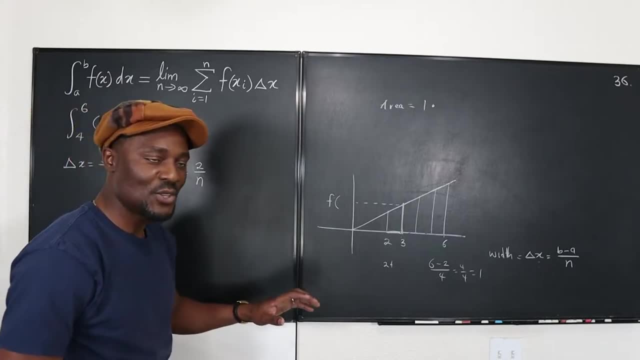 b is 6 and a is 4, so here it's going to be 6 minus 4 divided by n, which is 2 over n. This is a very important thing you just did because it's part of what we need. The next: 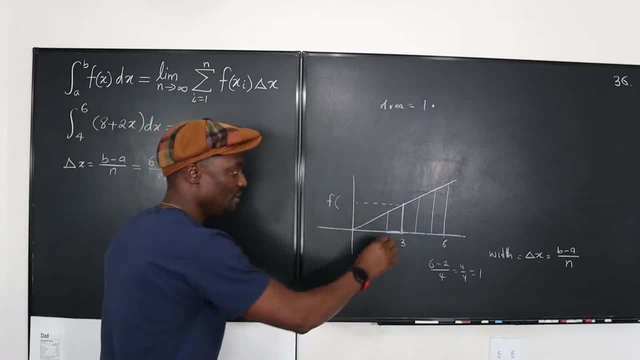 thing that needs to be modified. Oh, by the way, let's go here. So, in order to find this height, the height is going to be here, three, but remember, we don't know what we don't know. there's a three. the only thing we know is two, and we also know that every gap is going to be one one. 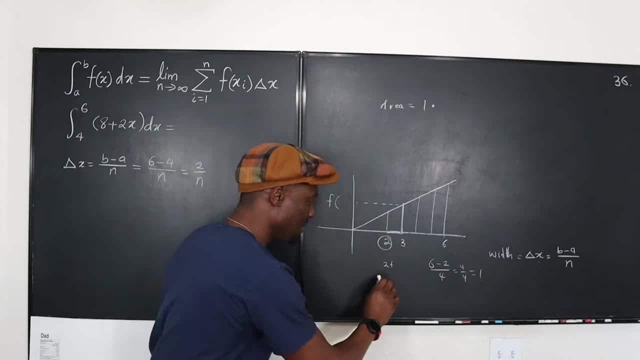 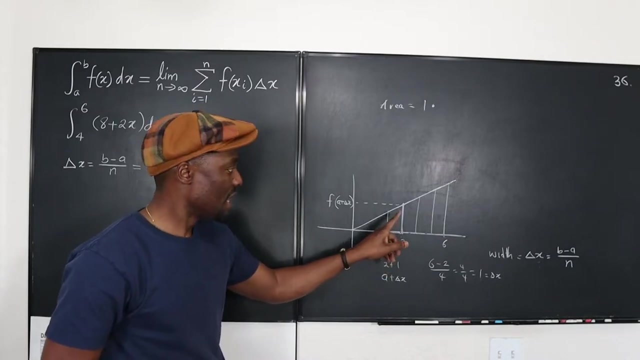 one. so to get to the first point, it's going to be the beginning: two plus one. remember this. two is your a and what is your one? again, it was our delta x, so it's going to be a plus delta x. that is the first point: a plus delta x. so i found the area of the first rectangle. i go to the next one. i know. 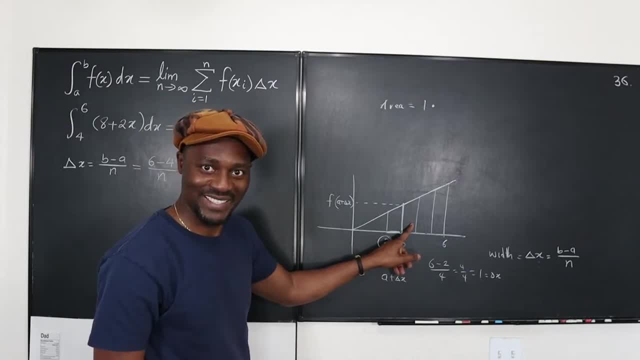 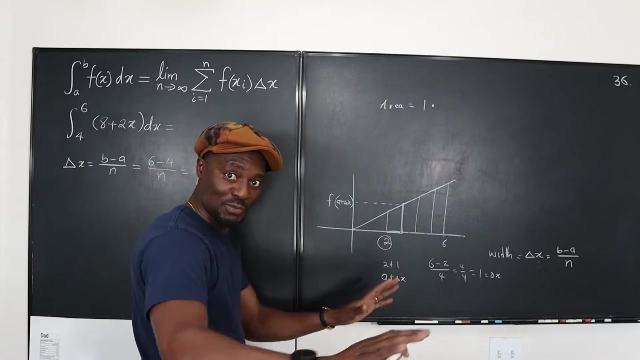 you're saying it's not a rectangle, but we have to take it as a rectangle. okay, because it's an approximation. we go to the next rectangle. we want to find the area of this rectangle. well, since we're using the right hand side and remember we didn't know this number was three. okay, let's assume. 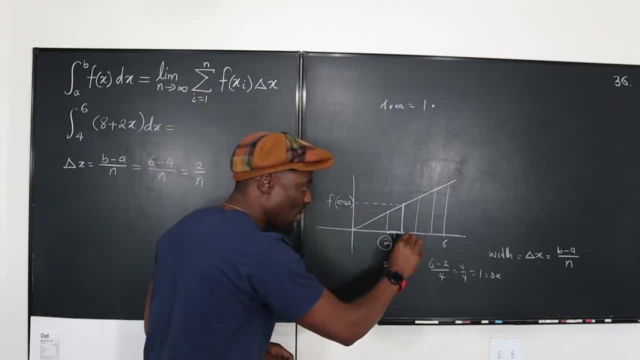 because it's not part of the question, but we know this is a three, so we're going to take it as a one. we know this is one. we know this is one. we know this is one. remember that one is delta x. so definitely, if i want to find the width of this, it is still the same. so the area is the width times. 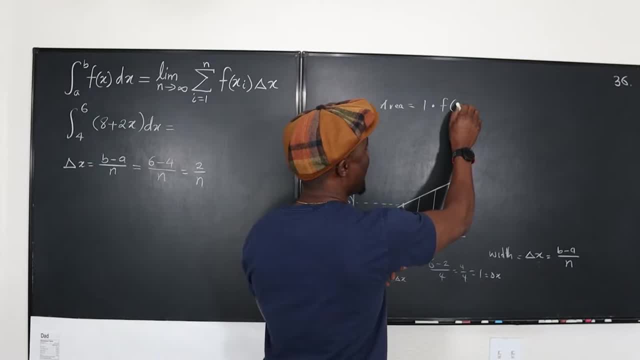 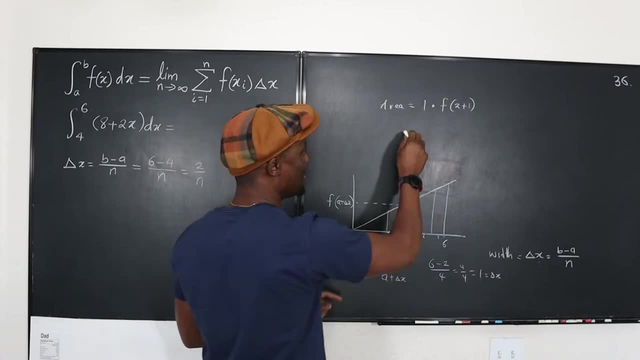 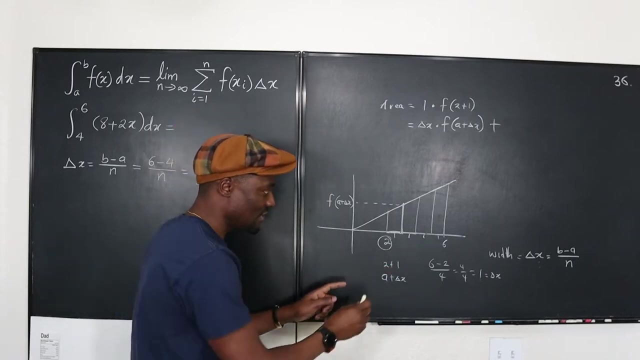 the function evaluated at two plus one, which is obvious. it is this times two plus one, okay, which will have the same form as remember, this is delta x times f of a plus delta x. That's the first area. Now we need to add the second area. The second area is: 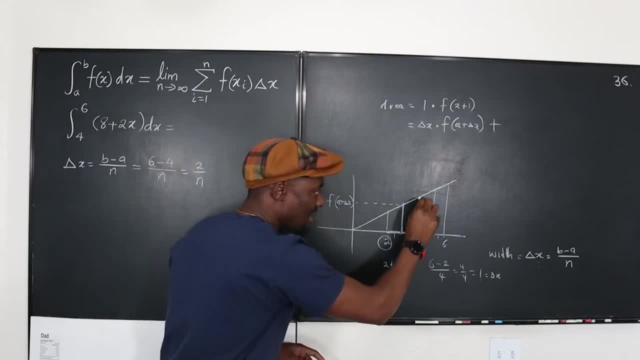 going to be this same area times this height. What is this height? If you trace it all the way here, it's going to be f of a plus. well, there are two. you have to add two delta x's to get there, So you 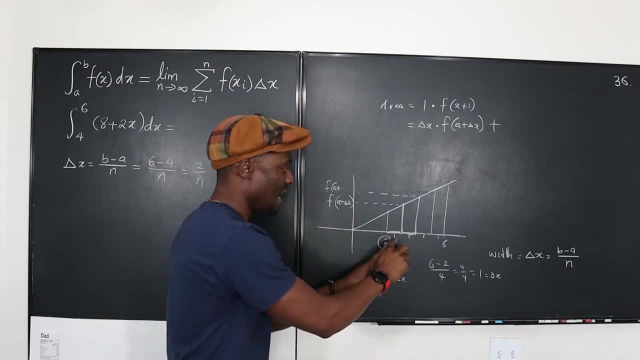 start from two, that is, your two plus delta x, plus another delta x. so that's going to be delta x times two, Okay, And then we can go on again, Delta x times three, delta x times four. If you add two to delta x times four, you're going to get to the end of it. So you notice that the next one. 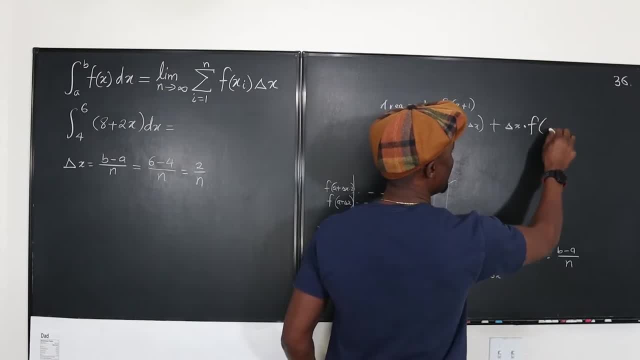 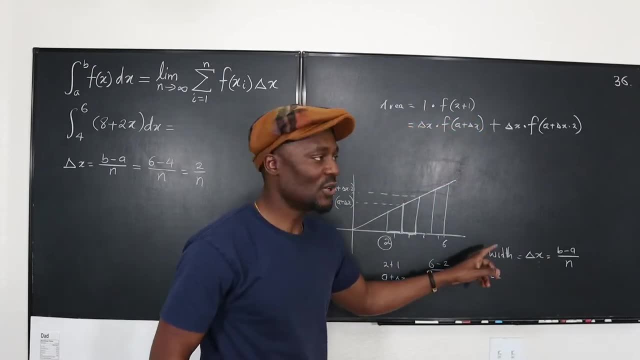 is just going to be delta x again, times the function evaluated at a, plus delta x times two. Well, if there are seven rectangles, you're going to keep adding until you get to delta x times seven. So you're going to get to the end of it. So you're going to get to the end of it, So you. 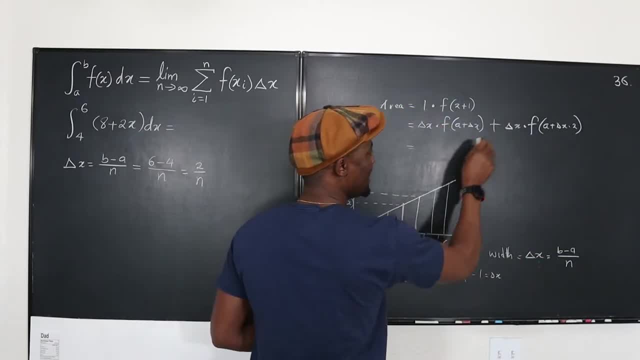 watch this, You will notice that everything has delta x, and then you're going to have f of a plus delta x. Look, f plus a times plus delta x. delta x, two delta x, three delta x, four delta x. How? 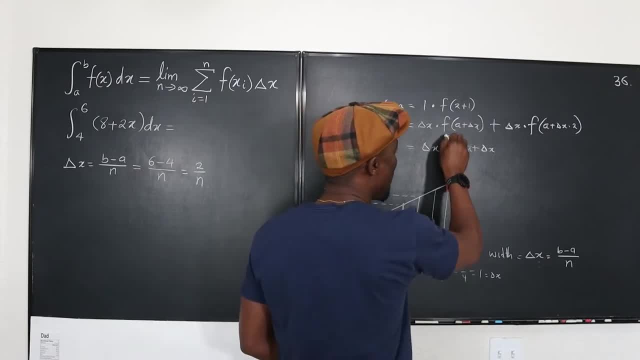 many delta x's? Well, it depends on how many, So we can just add all of these. This is the reason why the sum is so important, So we can just add all of these. So we can just add all of these. 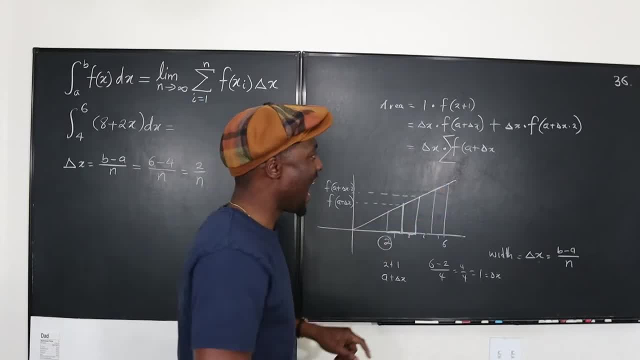 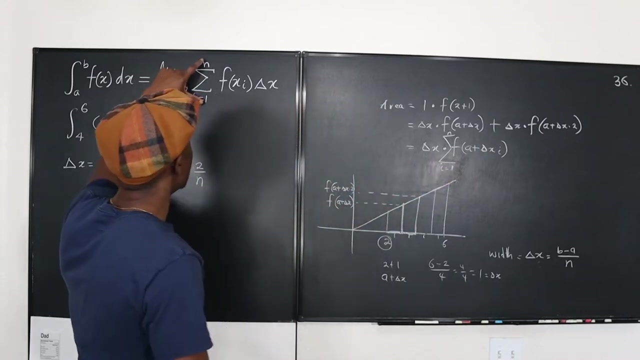 The sum is there. Okay, So we're going to add all the delta x's, where the first delta x will be multiplied by one, and you keep going until the number that you desire. That's where this sign came from. You see, this delta x is constant because it's a constant answer. It doesn't change. 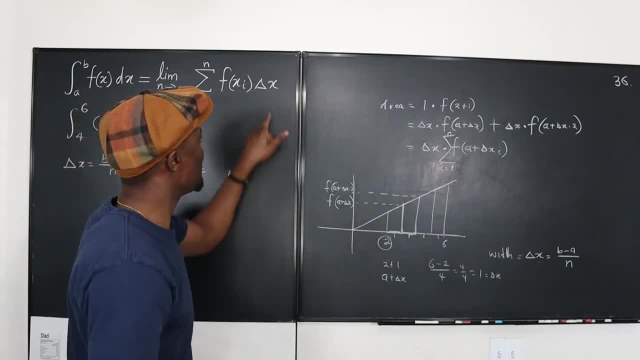 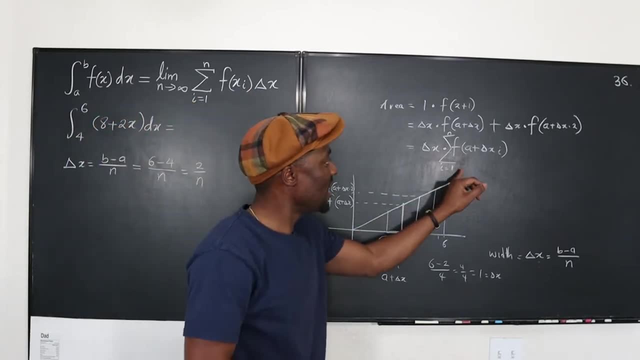 You can put it inside, You can move it to the back, It doesn't matter. So this delta x could actually be here. The only thing changing is anything that has this: i, because you have one, two, three. So remember in your head: i means one, two, three, four, five, six to infinity. i squared means one. 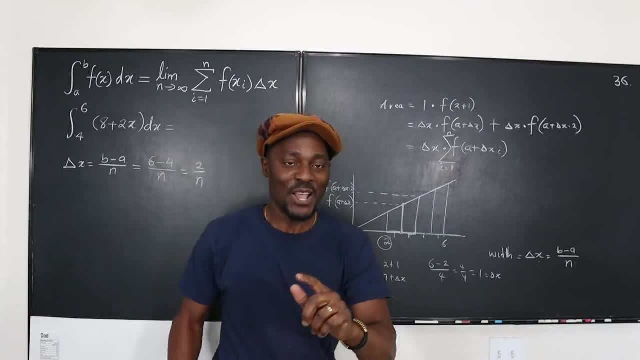 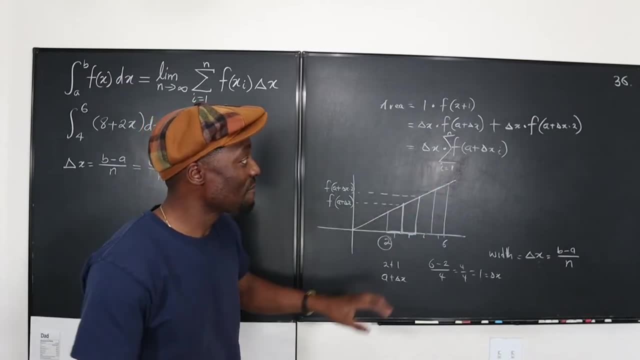 squared plus two squared plus if you put the sum beside it. Because with this idea you're good, You're good to go, Because now we now see that that thing in the middle of the triangle is going to be four And therefore what we have now is we have this x squared times the number of x squared. 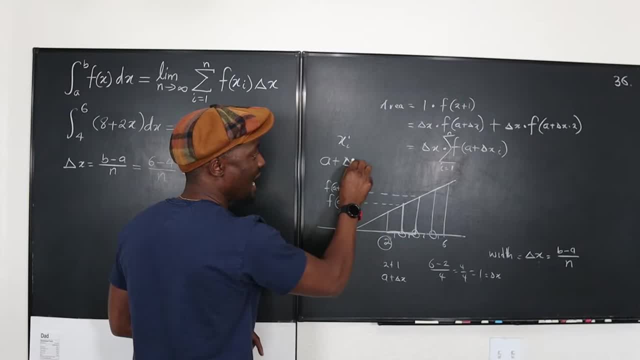 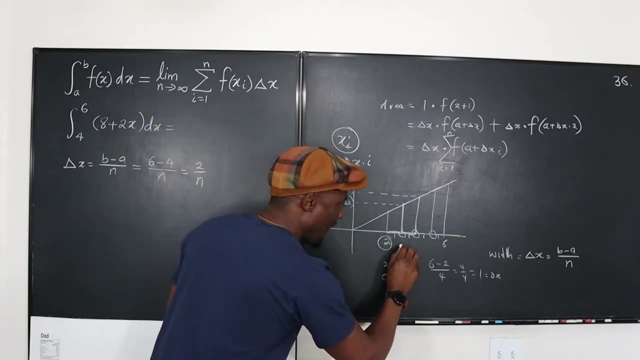 times the number of delta x's. Now, with this formula we called XI, which are? all these points are basically the beginning- A plus a certain number of delta x's- We just don't know how many. It depends on where this i is. So if it is i sub 4, then this would be A plus delta x times four. There will be four delta x's, Because I See this is X1, X2, X3, X4.. By the way, if you write it by the letter X in the middle, it's just X1.. X2, X3, X4.. 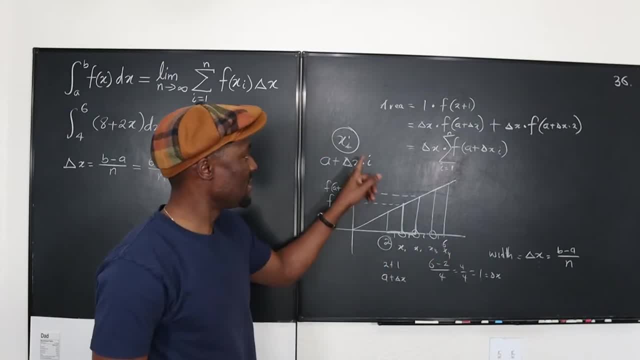 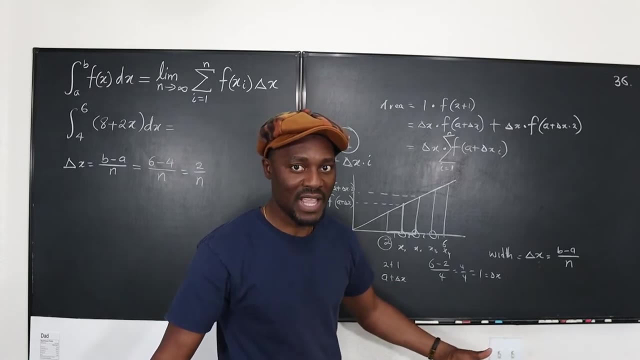 as you can see, for this example, x4 is basically a plus delta x times four. what's our delta x is one. we calculated it to be one. one times four is four. what is a two? two plus four gives you six. so if you had one million rectangles, that's the same idea and that's why we said we're just going. 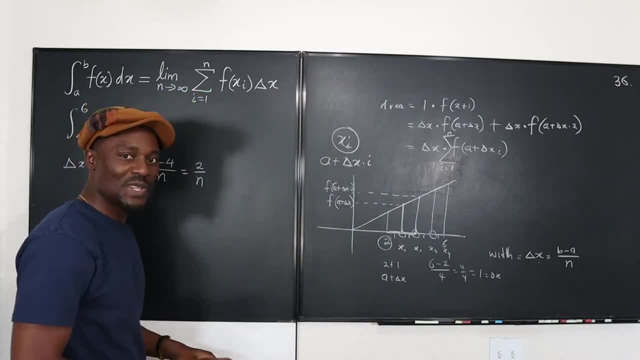 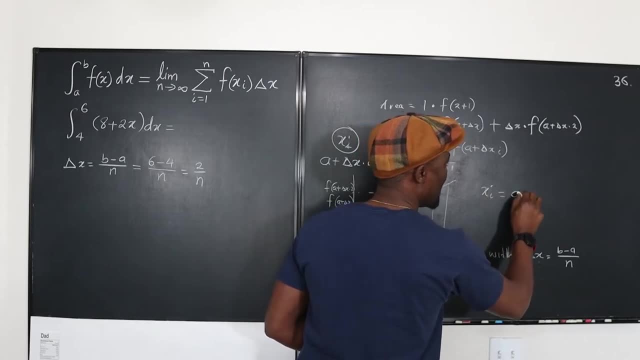 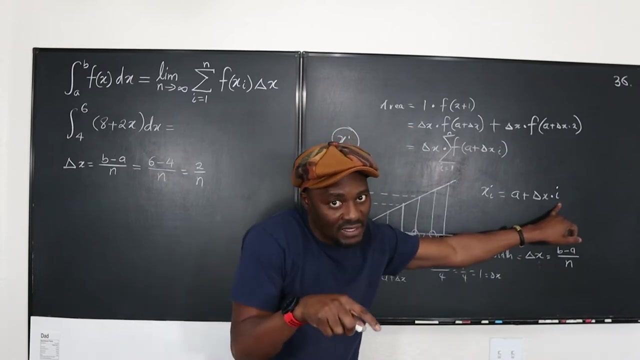 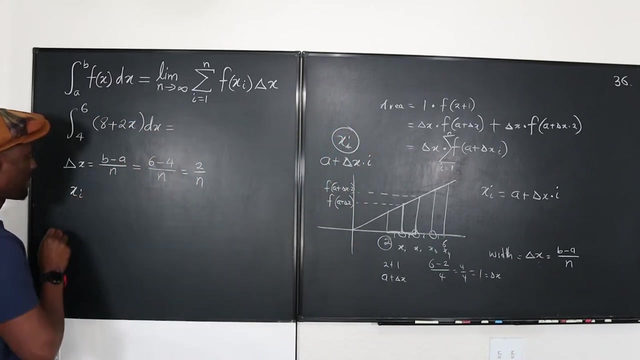 to generalize it, and that's the idea that you have. so the next thing you want to prepare is what your x i is. so generally, your x i is equal to a plus delta x multiplied by i. this i is not a subscript, so it's not delta x i, it's delta x times i. so here i'm going to write: x i is equal to a plus delta x. 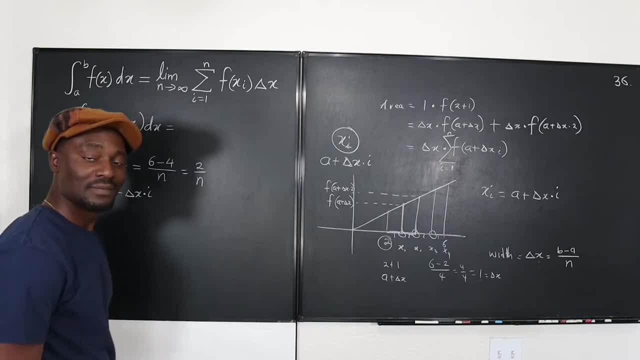 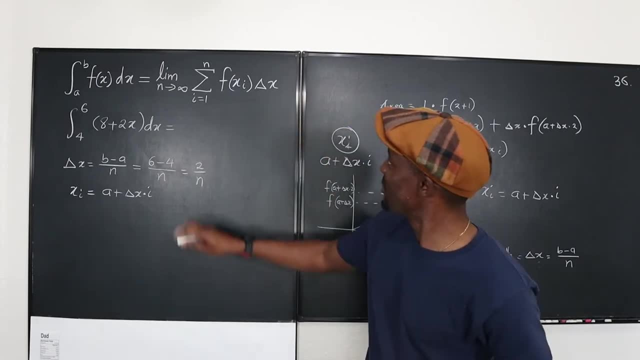 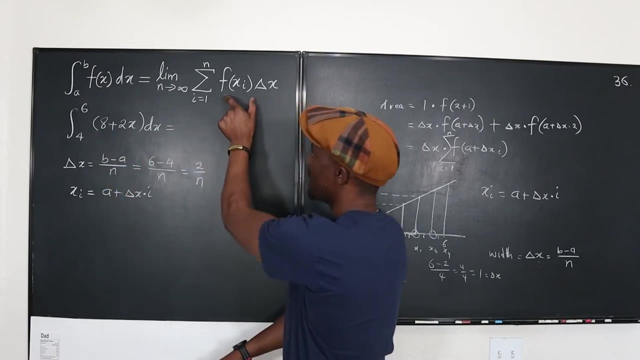 multiplied by i, and this is the most work you need to do, because now we just have to go back and do this and say that this integral- remember- this- is the function we're given. so when you want to integrate this function here, this is what you're going to write to replace this. but instead of writing x, this is what you're going. 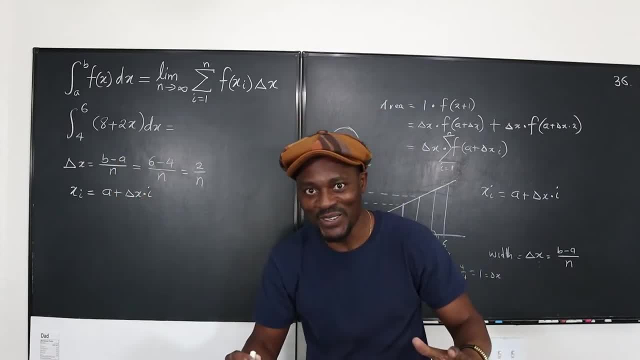 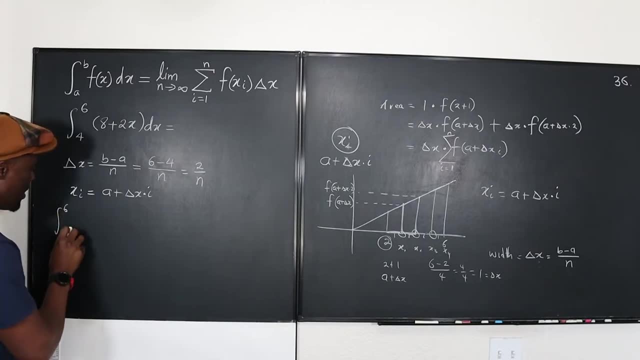 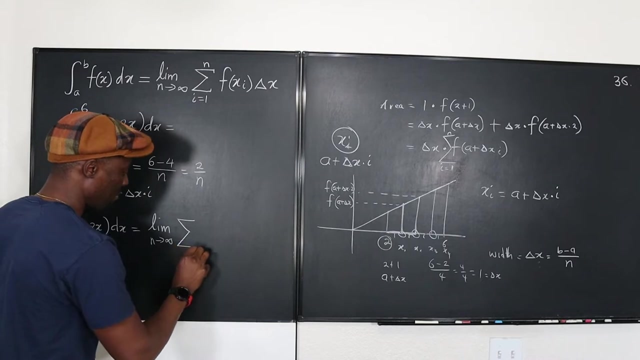 to write there and we just do some algebra. okay, just follow me. okay, so let's go. so here we have. we say that the integral from four to six of of eight, plus two to x, dx, will be equal to the limit, as n goes to infinity, of the sum from i equals one to n of f of. 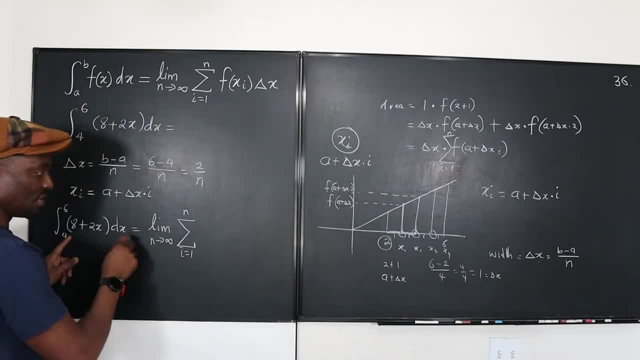 xi, f of xi we're going to replace- remember this is the function. it's going to be 8 plus 2. instead of writing x, we're going to be writing a plus delta x times i. but we know what a is, so let's just quickly write it out. 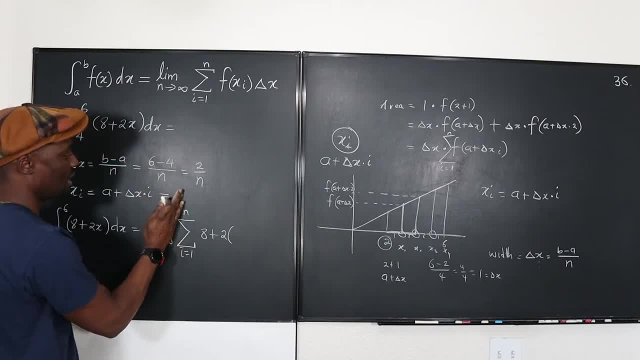 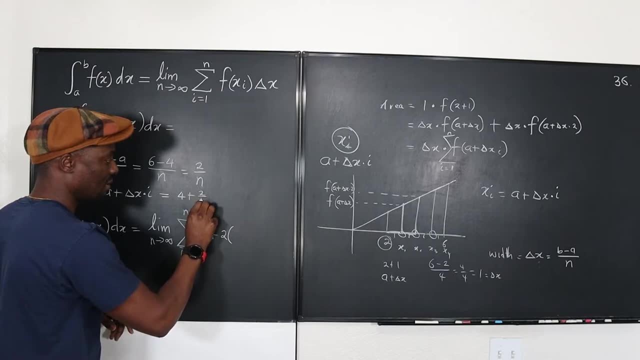 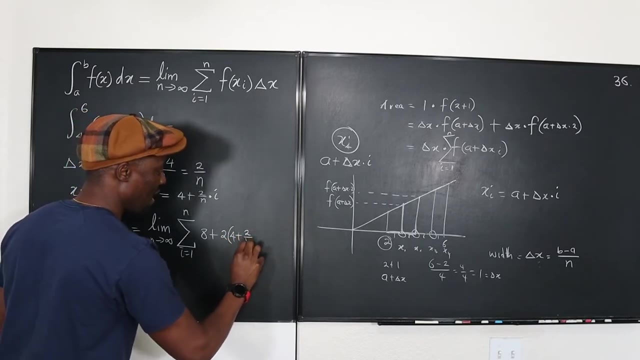 this is equal to 2. oh, it's 4. actually, it's going to be 4 plus what's our delta x is 2 over n, multiplied by i. so it's going to be 4 plus 2 over n, multiplied by i. okay, and multiplied by delta x. 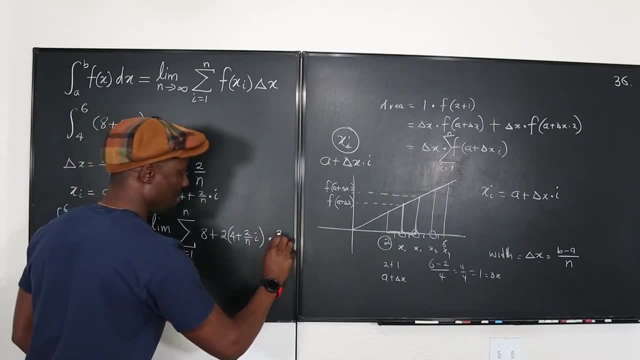 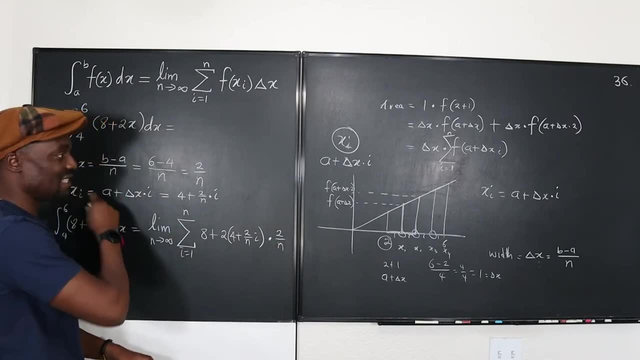 we're going to multiply again by what's delta x, 2 over n? okay, remember where i told you that this is a constant and that's why we're going to move it to the back of the equation. we're going to move it to the back of the equation, we're going to multiply it. so the delta n- 2 over m over n, which? 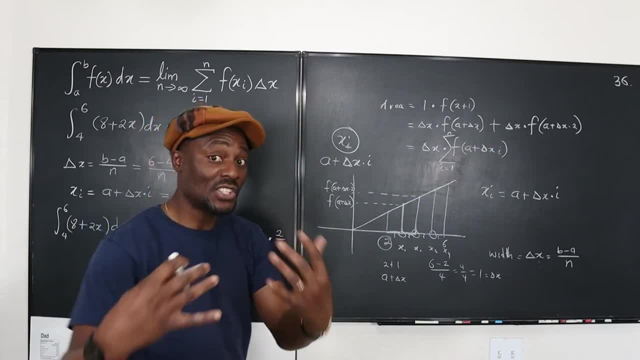 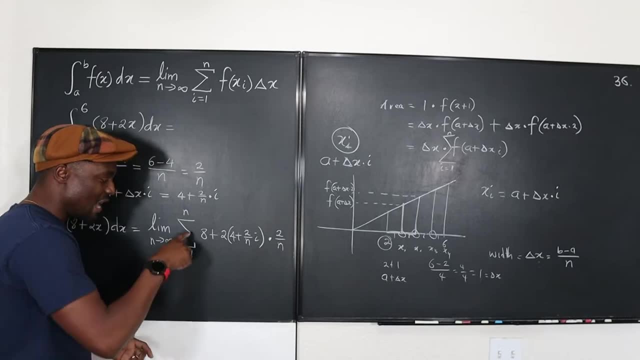 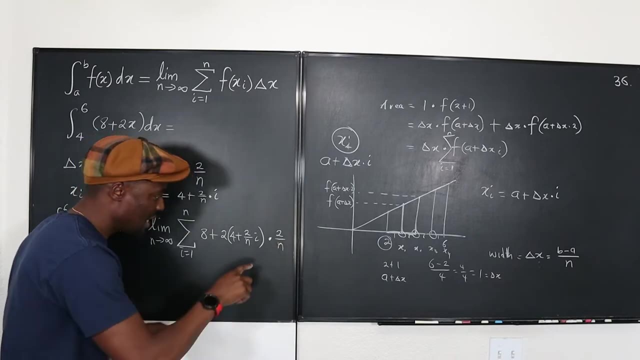 is our delta x is a constant. we could have moved this all the way. that's why we put it in the back here, so it's safer. this is a recommendation. i recommend that you move it to the back because it's a constant. now, look, i know, you see i. you see n and you see n inside here. the only thing changing. 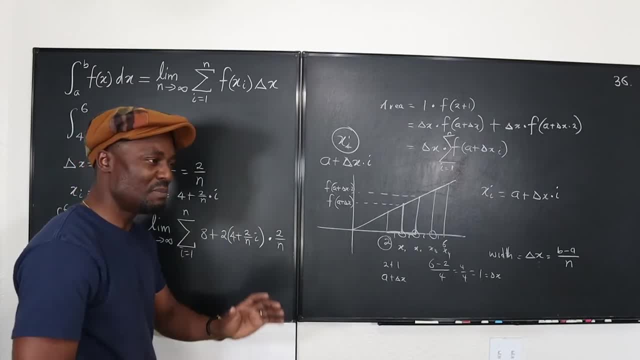 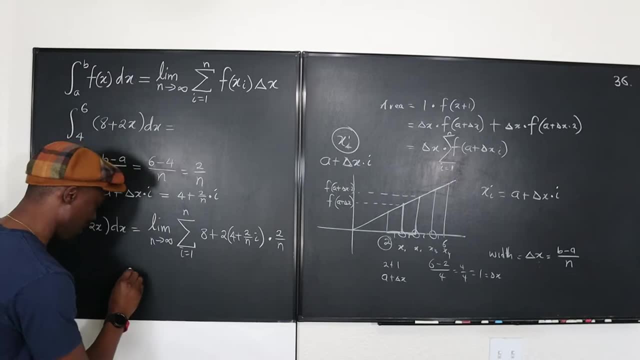 here is i. nothing else is changing. everything else treated as a number, as a constant. so if it behaves i, it's a constant and you can move it to the back of the summation sign. okay, so let's clean this up. this is going to be the limit, as n goes to infinity. now i'm going to try to clean this up. 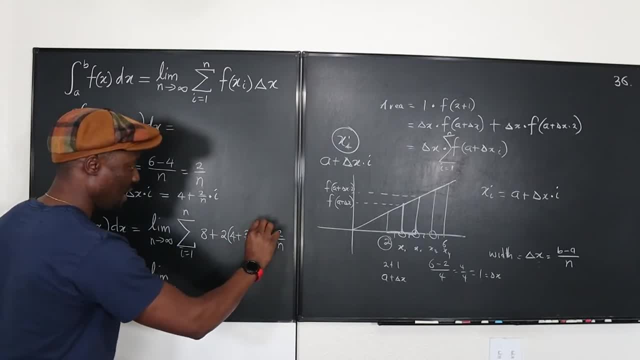 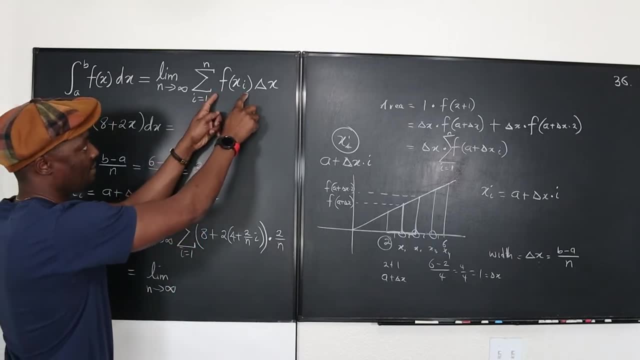 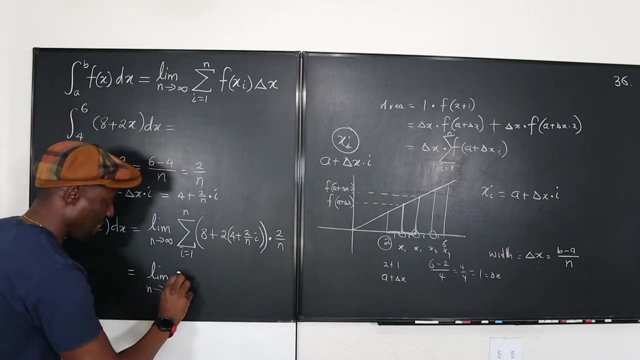 see 8 plus 2 times. let's leave this out here, okay? oh, all of this will have to be multiplied, so there's a parenthesis here. okay, you get it. so remember, it's f of x i times delta x, so that's f of x sub i. so now i can move this to the back, like i promised, and then this is going. 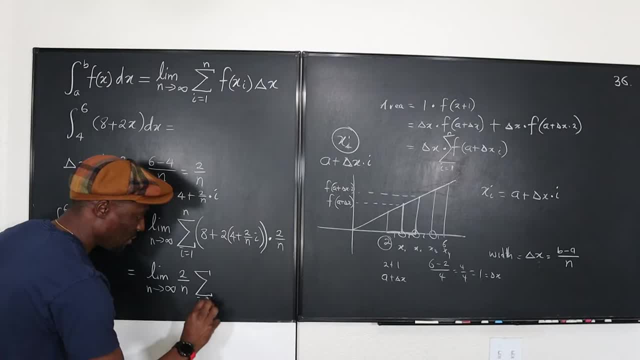 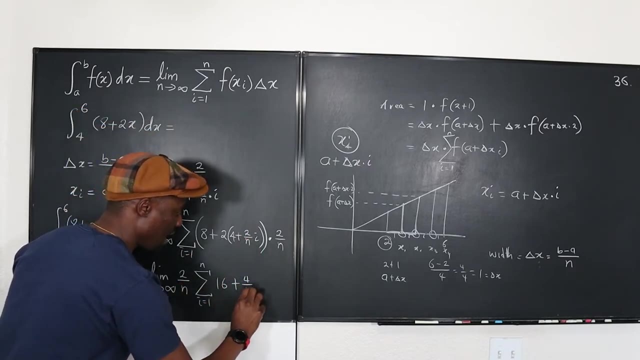 to be: the sum from i equals 1 to n of. if you clean this up, this is going to be 8 plus 8, that's 16, okay, and if you multiply 2 by 2 over n, it's going to be 4 over n over n i, okay. 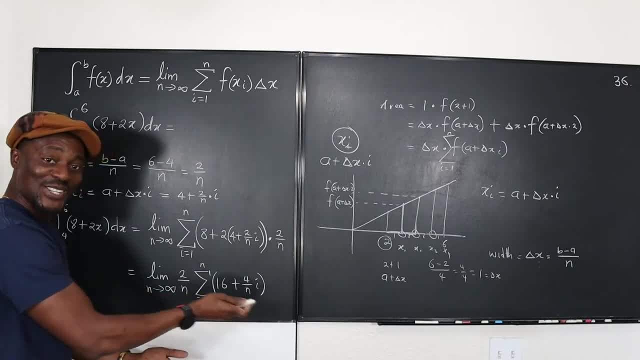 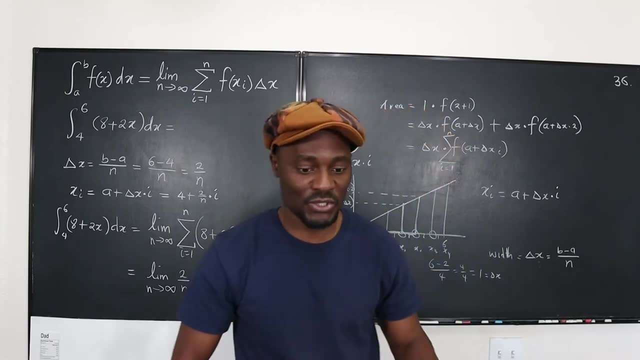 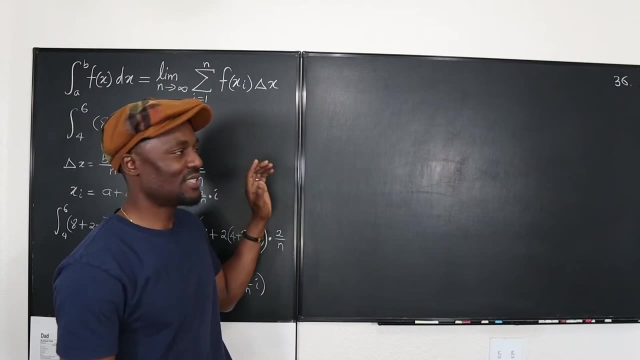 that's it. we just need to do this now. if you didn't do this in your pre-calculus days, maybe this is why this might be tough for you, but it's not difficult. just watch the process i'm going to go. let's get rid of. by the way, before i started the video, i quickly did the integration of this. 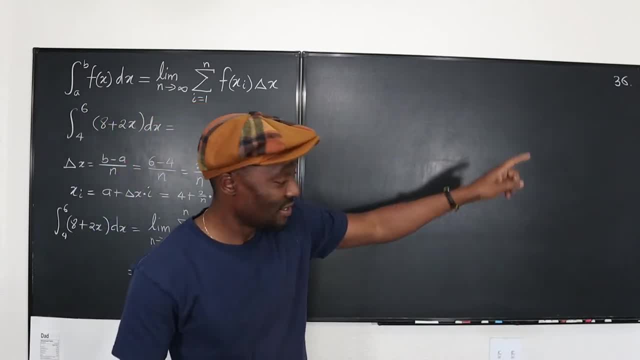 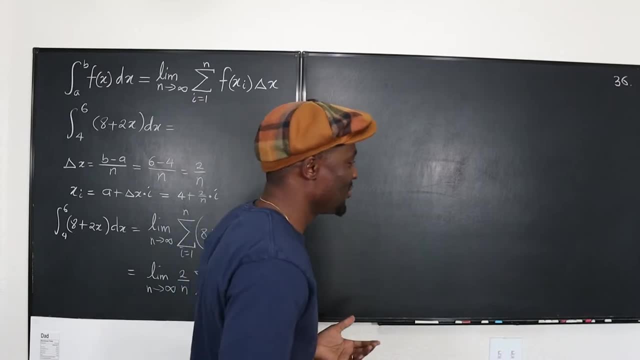 just the normal integration. i know we should get 36, so that's why the number 36 is sitting there. so if i don't get 36, you know we've messed up. okay, and you didn't say, hey, you're wrong. well, you were just watching, you didn't correct me. 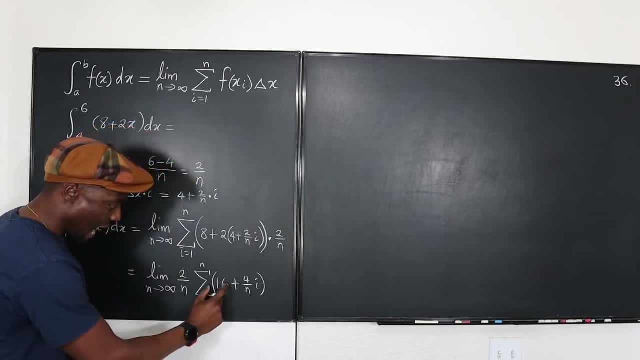 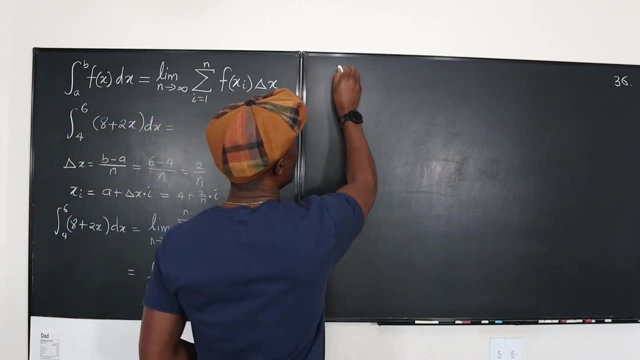 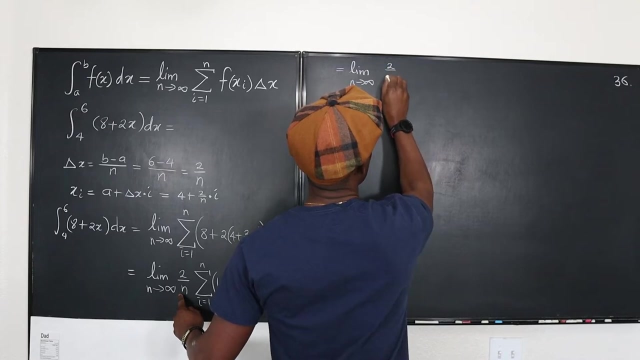 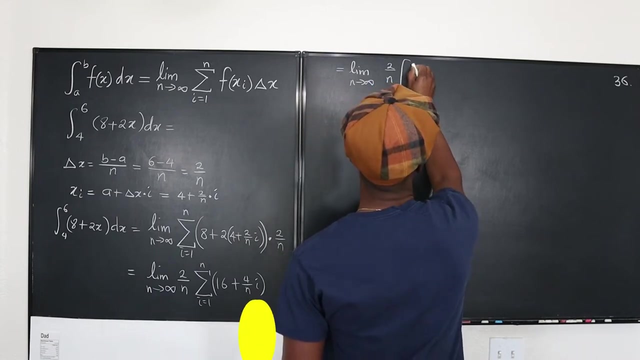 this is what we have at this point. so now i can separate these two. watch, i can separate these two. so what i have now is equal to the limit, as n goes to infinity, of 2 over n. now i'm going to separate these two, so let's make this giant parenthesis. so this is going to be the sum to infinity. 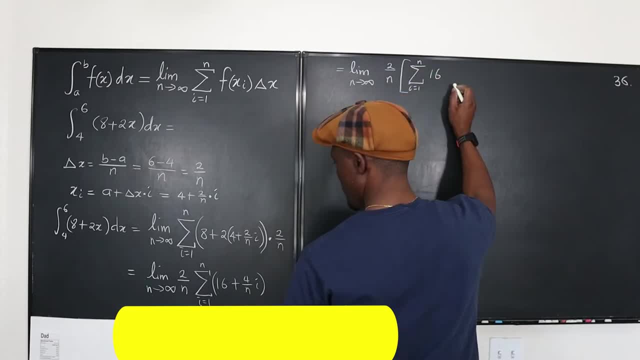 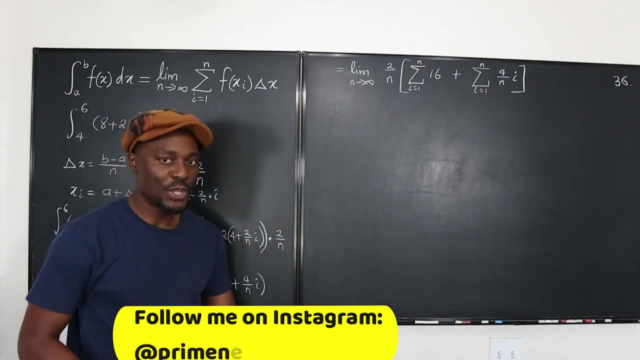 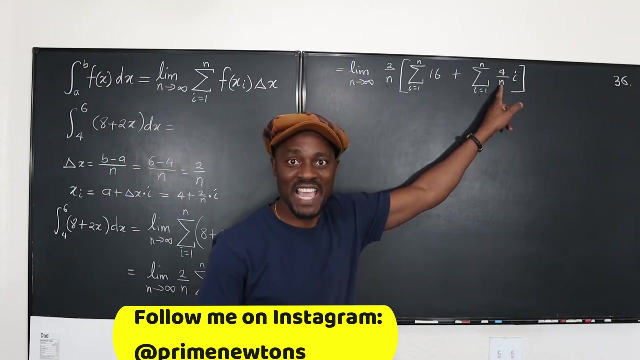 from i equals 1 to n of 16, plus the sum to infinity of i equals 1 to n of 4 over n i. okay, now, if you recall what i said, if it doesn't have an i, it's constant. you see this, 4 over n, treat it again as a. 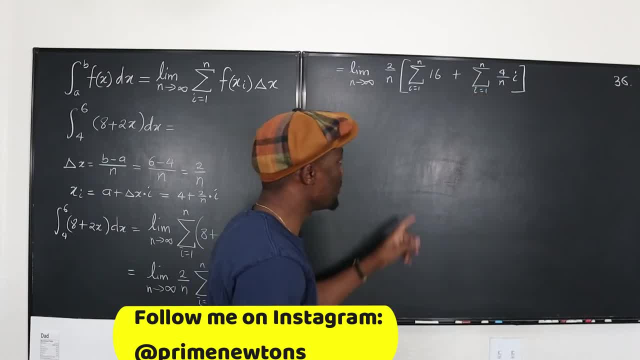 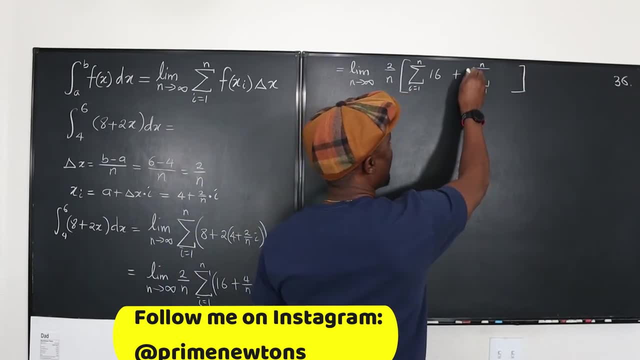 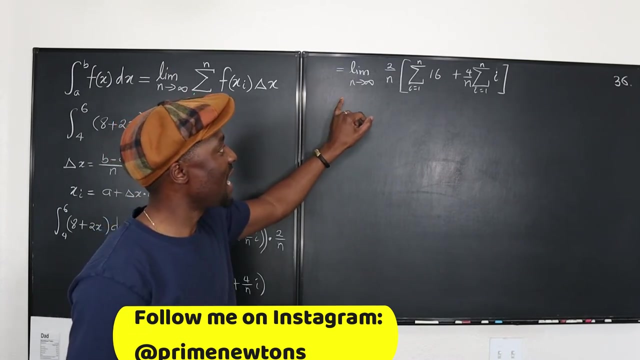 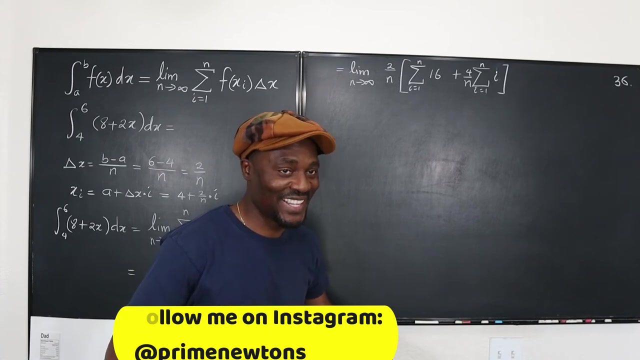 constant move it to the back. so i'm going to just move it without rewriting. so we're almost at the end of what we're doing, because now, how do you? what does this mean? okay, so that's another thing. this is pre-calculus. now it's no longer calculus. okay. 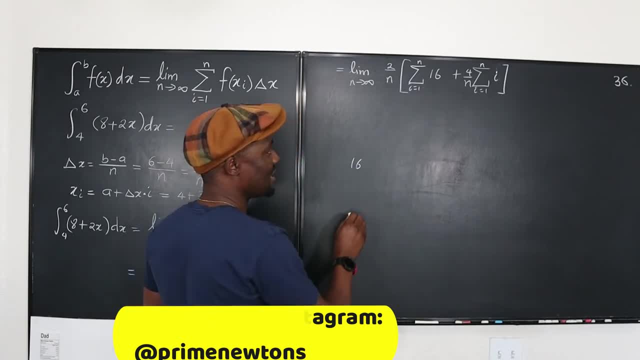 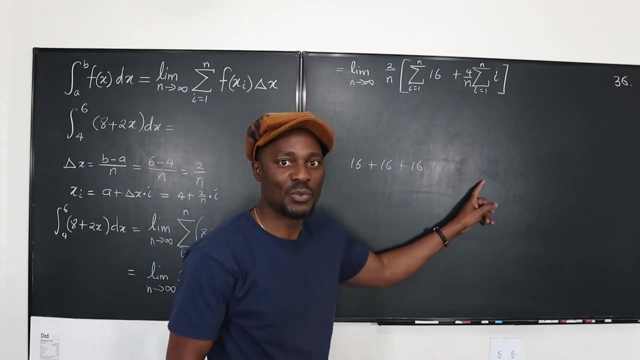 what does this mean? this means add 16. the first 16. see, this is a constant. add it to another 16, keep adding 16, starting from the first one to the nth one. so let's say i'm doing it 10 times, then this would be 16, 10 times, which is 16 times 10, which is 160. 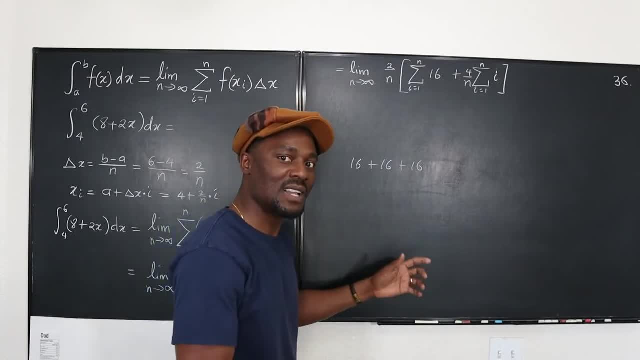 if i'm doing it n times, it's going to be 16 times n, which is going to be 16. n makes sense, right? so if you're doing it four times, it's going to be 16 times 4, which is going to be 70. 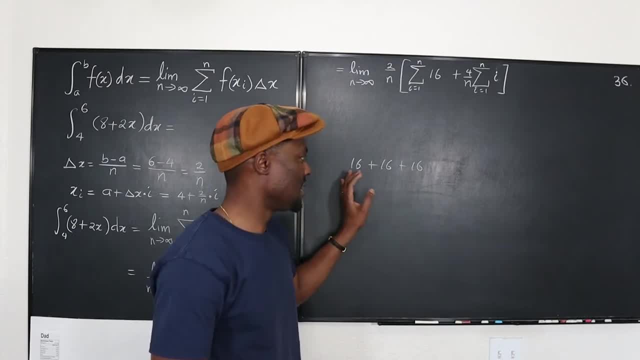 which is going to be 64. okay, or you just say 16 times 4, or 16, 4 times. so that's the meaning of this expression. so if you struggled with this, it's because you didn't know what this meant. but now that you know, we're going to have the limit, as n goes to infinity, of 2 over n. now we're. 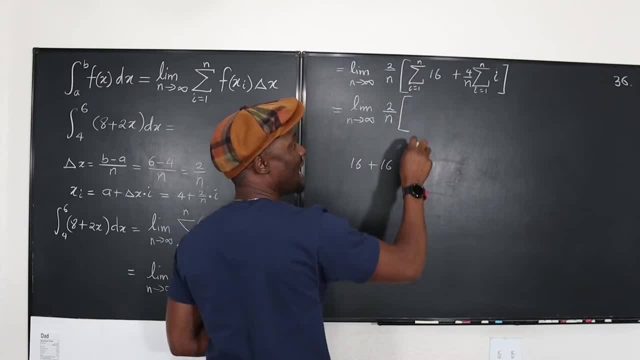 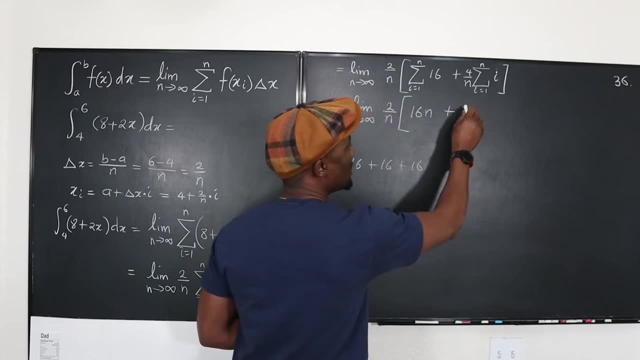 going to still have this. this means 16 n times, because you're starting from 1, so it's going to be 16 n plus if we do this one, this is going to be 4 over n. what does this expression? so let's go back to this expression. 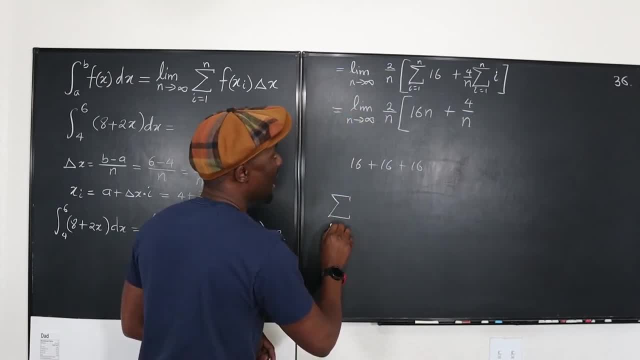 again. okay, this means um from i equals 1 to n of i. now this is the one. this is slightly different because you see, 16 was not changing. there's no i is attached to it. but in this case we are saying i is changing from 1 up until n and you're adding everything together. so this simply. 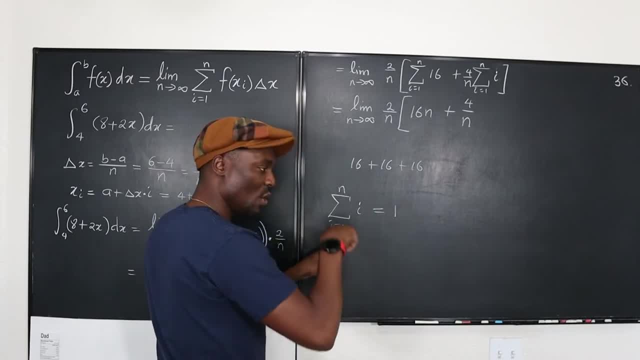 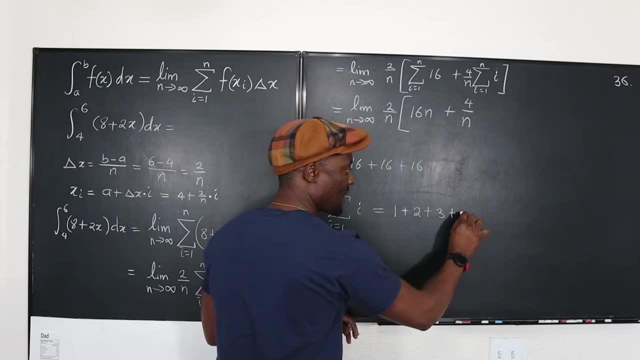 means if you start i from 1, it goes to the next number. remember we're always adding. this means sum. keep adding plus 2 plus 3, plus 4. you keep going let's. let's say we stop at 10. let's say n is 10.. we know n is going to infinity, but i want to use this to explain the concept. so 1, 2, 3, 4, 5, 6. 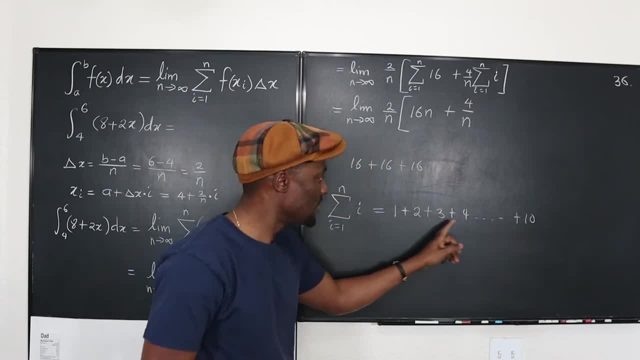 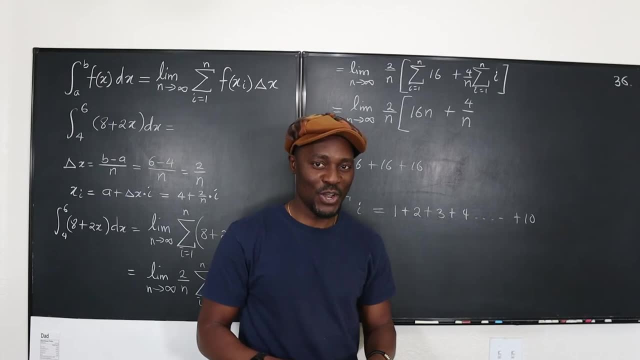 7, 8. let's say we stop at 10. how do you add 1 to 10 the fastest way? if i asked you now to add 1 to 10 the fastest way- yeah, i know. what you know is you're going to say: i'm going to add 1 to 2, then to 3 and then to 4. 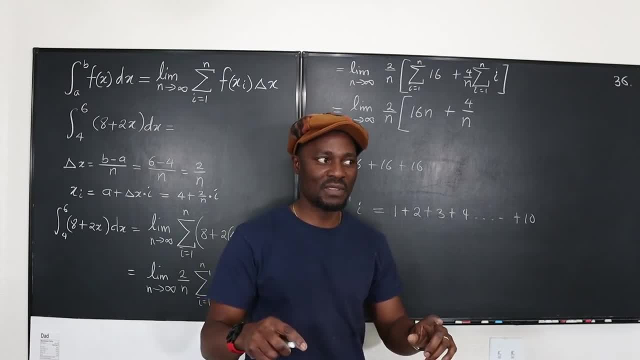 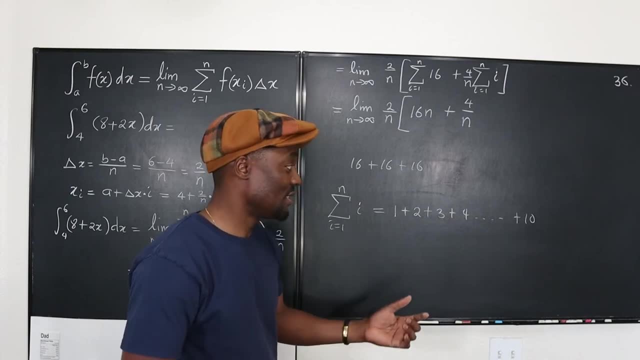 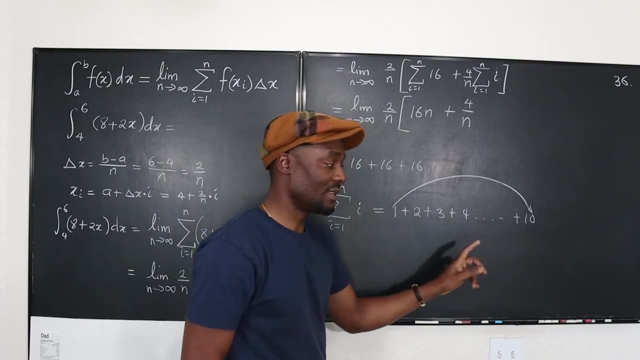 that's 10, then to 5, that's 15, then 21 plus 7. that's going to be. you see, you start thinking and doing arithmetic, but you don't know. you don't have to if you know the formula for it, which is simply adding the beginning to the end. 1 plus 10 is 11. 2 plus 9 is 11. 3 plus 8 is 11. 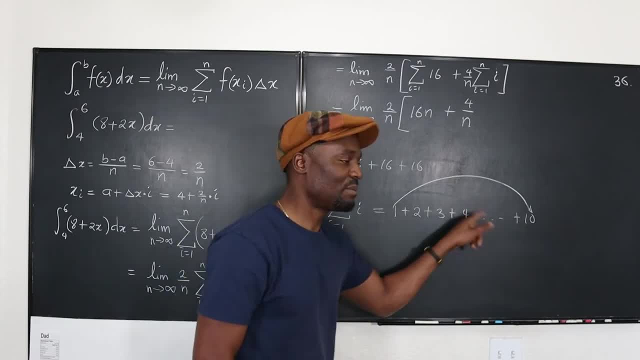 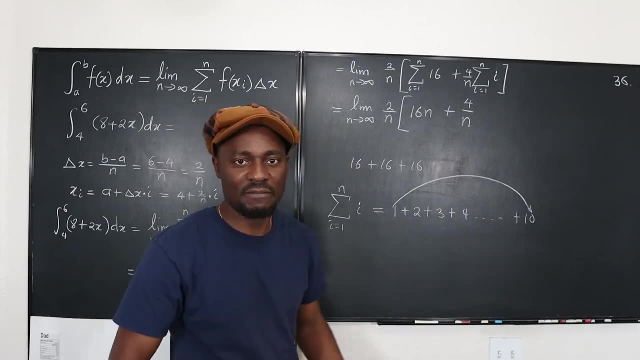 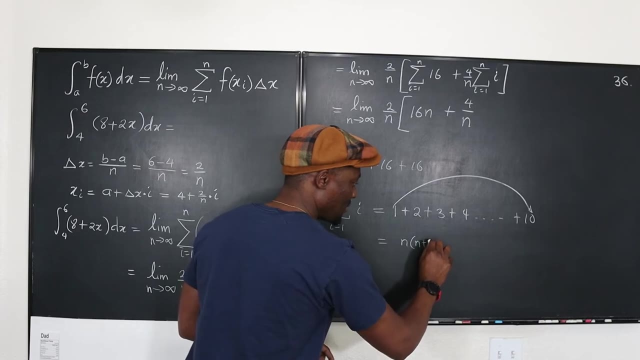 4 plus 7 is 11. 5 plus 6 is 11. did you see that? you've added all the numbers. you get 11, 11, 11, 11. how many places? 5 places. so this is the formula for this expression. it is the same thing as n times n plus 1 divided by 2 is the same thing as 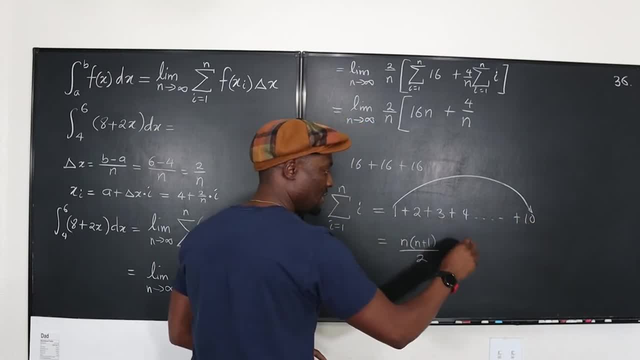 see, because you add it to 10. 1 to 10, it's going to be 10 times 11, divided by 2, which is 5 times 11, which is 55, the fastest way. so now you can add from 1 to 100. 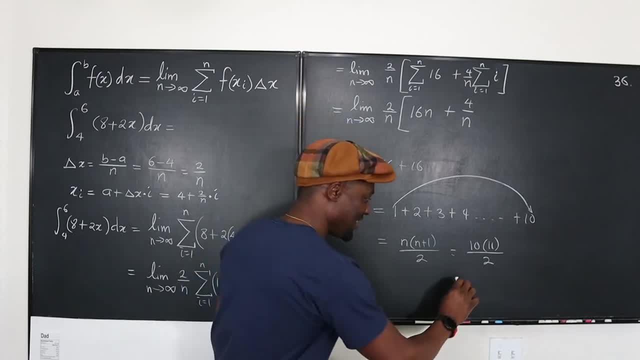 quickly remember, it's 100, so the first 100 integers is going to be positive integers is going to be 100 times 101. divided by 2, that's going to be 50 times 101, which is going to be 50. is it 50, 50? 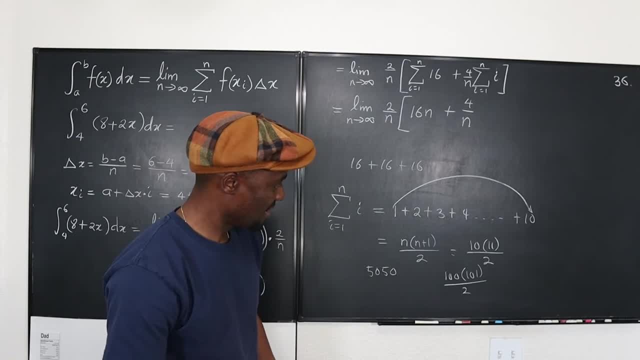 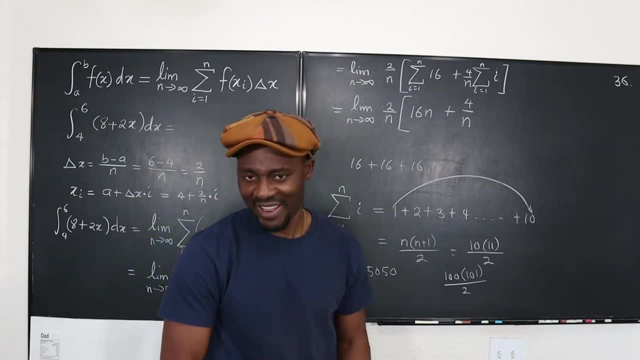 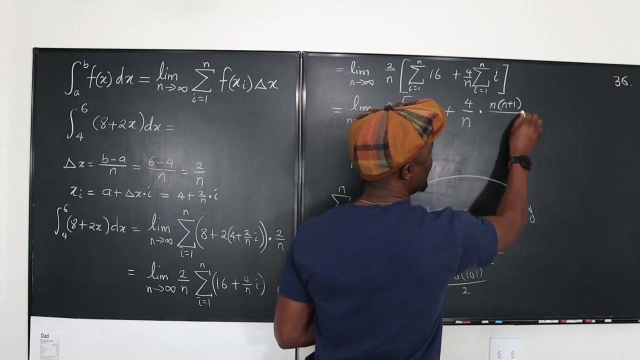 whatever, okay, is it 50, 50, 5500? leave it in the comment section. i don't care. whatever it's important is: you know the formula. this is what you now need to replace this expression- it is the sum of the first n integers- is going to be n times n plus 1 divided by 2. 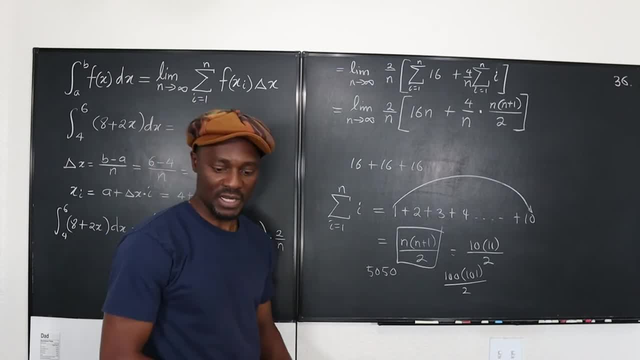 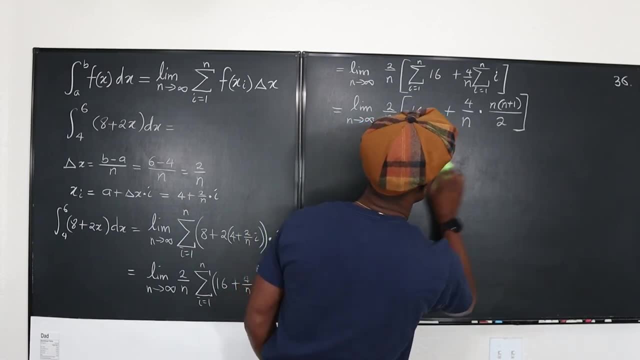 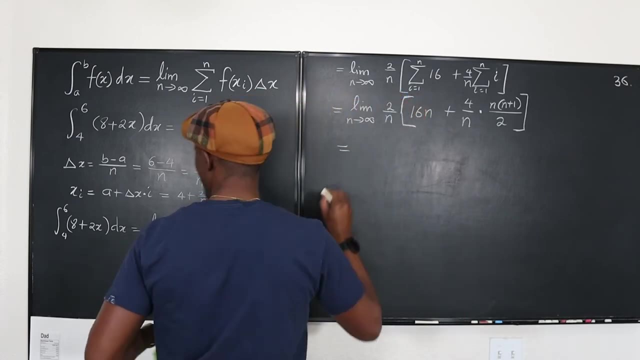 okay, i'm going to clean this up and we'll finish this. so we're at the end. actually, there's nothing more complicated. we've simplified every expression. i don't like this parenthesis, this bracket that i used. okay, that's better. okay, so what do we have now? 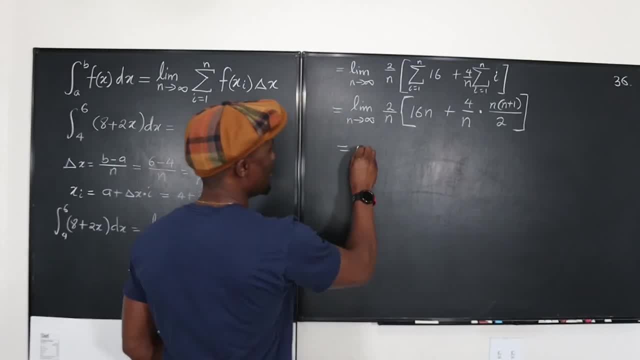 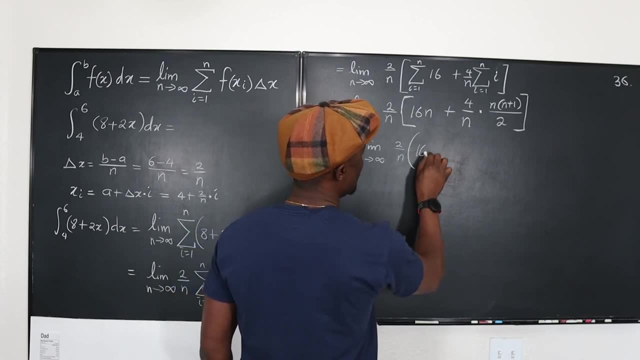 if i multiply now, i'm going to multiply. let's clean this up. okay, this is going to be the limit, and goes to infinity, of 2 over n, um times 16 n- sorry, i'm switching back to my parenthesis- plus, if we do this, this 2 will multiply this. and what would you get? you're gonna get um. oh, we'll divide. 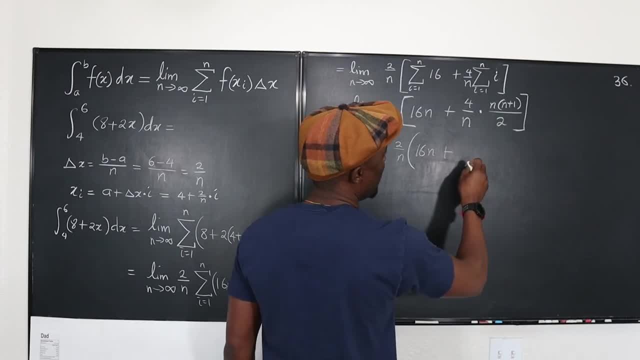 this, that's 2. this n will cancel this n. oh so iısı. the Vanessa is 5 Over. 2 is the end is the end of 9? N is that 2? this n will cancel this n. oh so I just have 2n. so this n cancels this n. this cancels we. 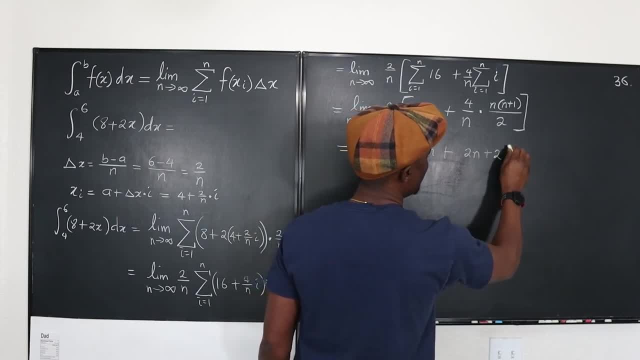 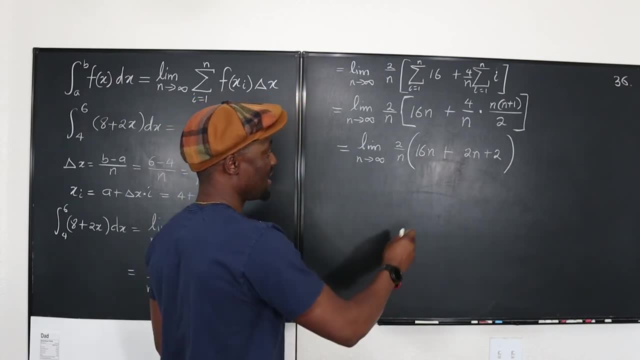 have 2 into n, so 2n plus 2. okay, I just have 2n plus 2 interesting. so now I can now take this and get rid of all the n's that are possible. so this is going to be the limit as n goes to. 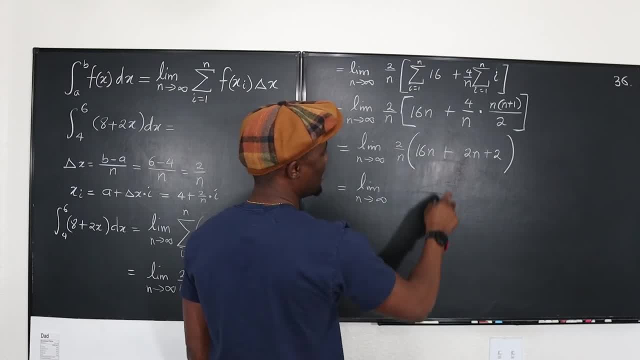 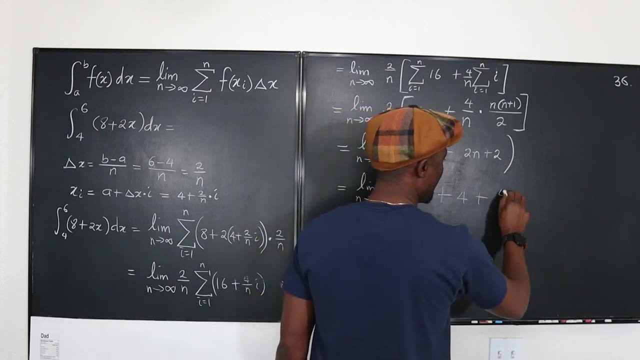 infinity of. if you multiply 2n by 16n, you 2 over n by 16n. you're going to get 32 straight plus. if you multiply this by this, this n will cancel this and you're going to get 4 plus. if you multiply this by this, you're going to get 4 over n. ah, now, if we take the limit, this is: 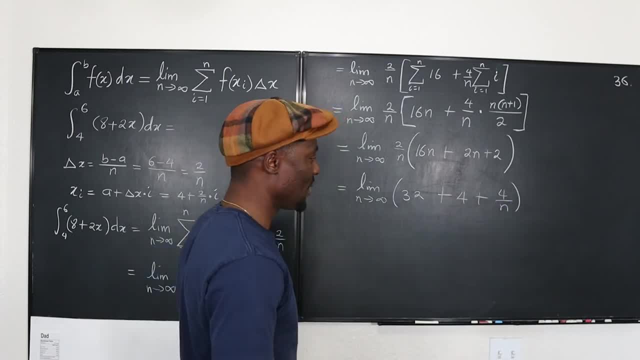 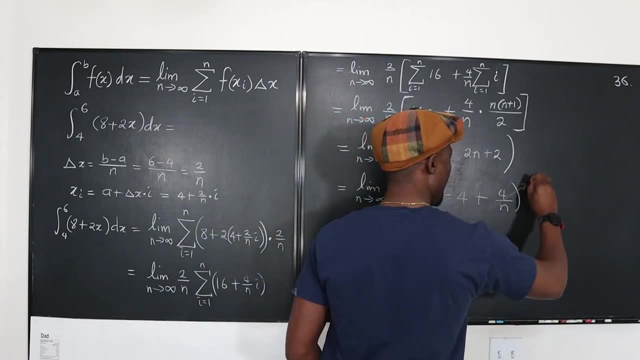 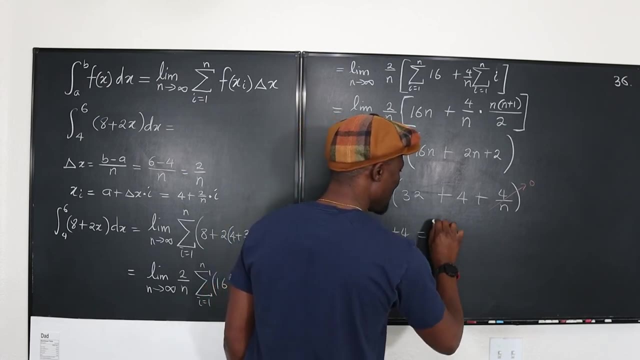 a constant. this is a constant and this is gonna go to 0. okay, so this is gonna go to 0, this goes to 0 as n goes to infinity right? so what do you have? you're going to have 32 plus 4, which is 36, which. 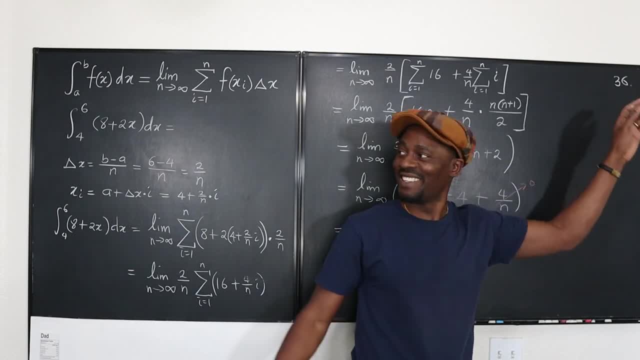 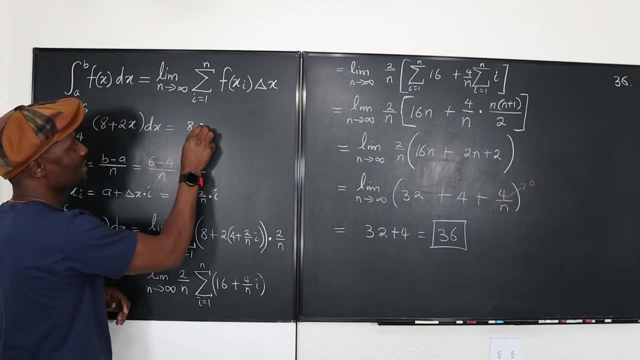 looks like what we got at the beginning. if you take your normal integration, that's what you're going to do. okay, let's finish that up. if you take the integration of this, you're going to get 8x plus x, squared, evaluated from 4 to 6. well, this is the same thing as 8 times 2. 6 minus 4 is going to. 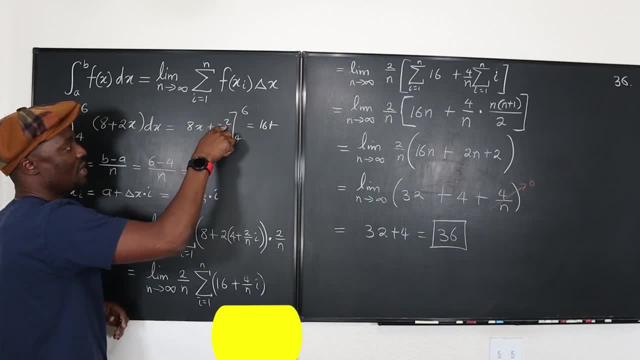 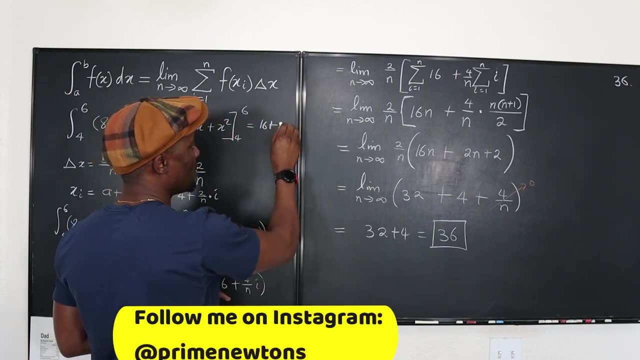 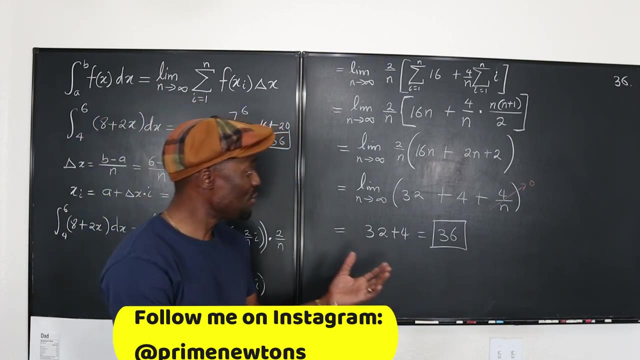 be 2, that's 16 plus. there's going to be 6 squared minus 4 squared. 6 squared is 36. 4 squared is 16. 36 minus 16 is 20. oh, that's 36, dude. well, that was what I did from the beginning. okay, I hope you. 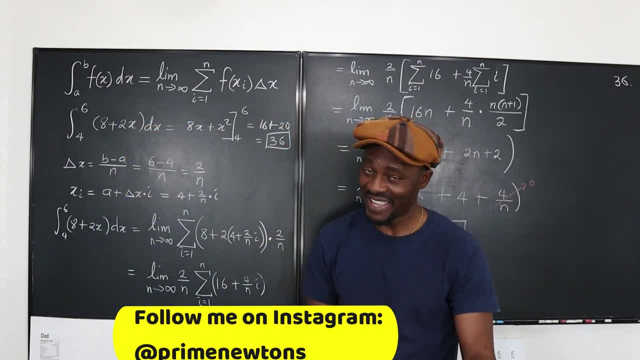 this made it a lot easier for you to understand. okay, I'll see you in the next video. don't stop learning. those who stop learning have stopped living bye.